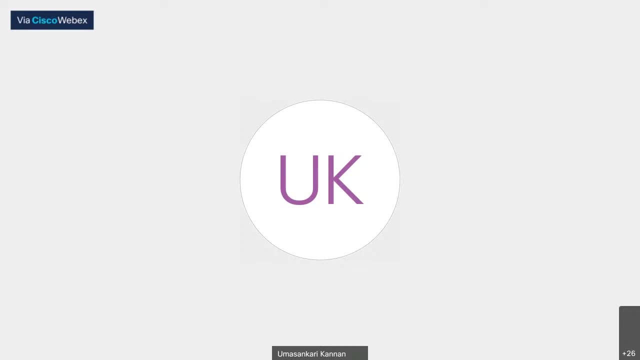 So good evening everybody. So this is the third module of the HB&I online course on nuclear science and technology. I am Dr Uma Shankari Kannan and I will be Thank you very much. Thank you, Yes, ma'am, we can see. 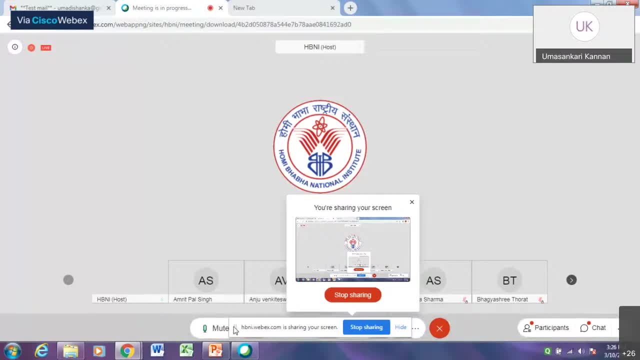 Yeah, but can you see my video? No, ma'am, you cannot see the video. You just need to open the. You have minimized the PPD. But can you see my video? No, ma'am, you cannot see the video. You just need to open the. You have minimized. 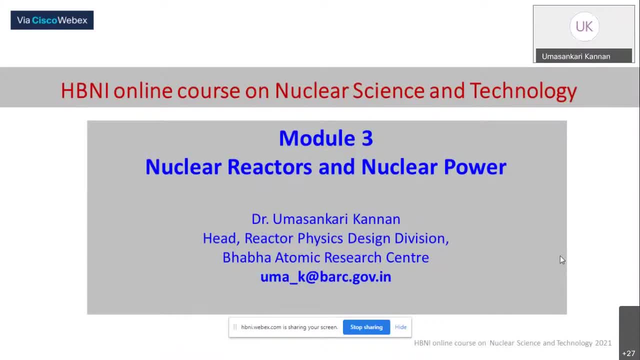 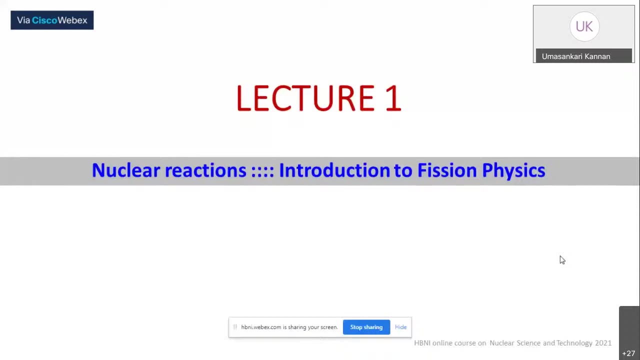 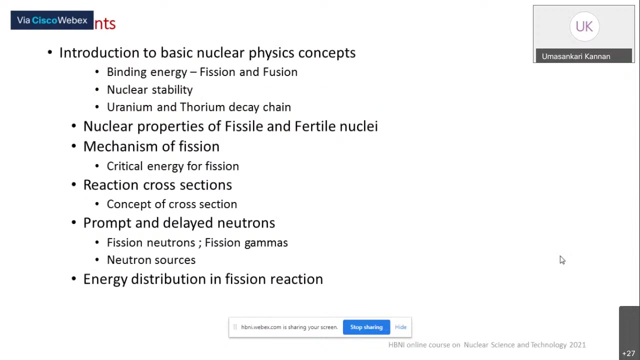 Okay, so I will start speaking then. This module is on nuclear reactors and Nuclear power- Previous lectures, which is, nuclear reactions, and I would like to introduce something on fission physics. The contents of this lecture would be some basics of nuclear physics concepts. 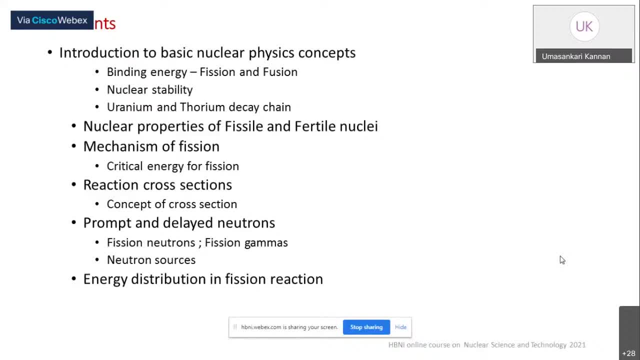 expanding energy, fission and fusion and what is nuclear stability. And I would like to talk something about the radioactivity decay chains of uranium and thorium. I would also highlight properties of material and exactly the mechanism of fission. 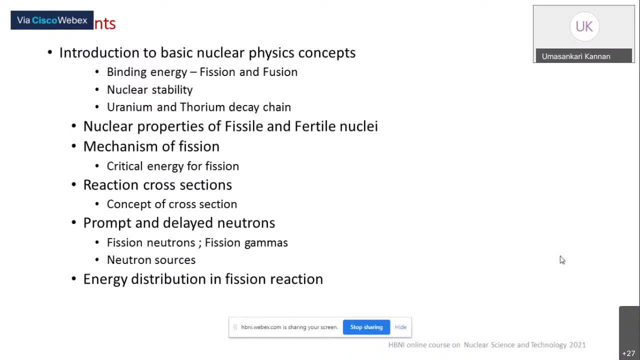 So there is some energy which is required for fission to take place. So I will be highlighting those aspects And then I will give a brief on the reaction. cross-section: What exactly is the meaning of cross-section? What is the meaning of? What is the concept of cross-section? 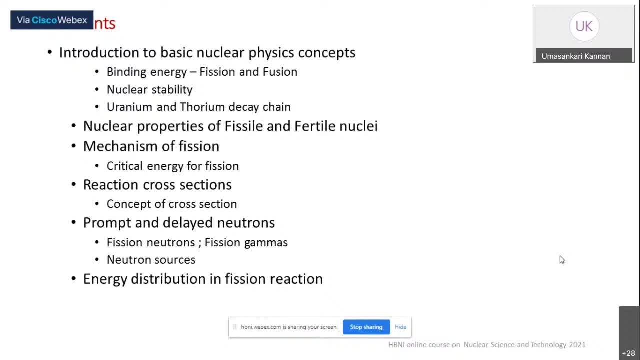 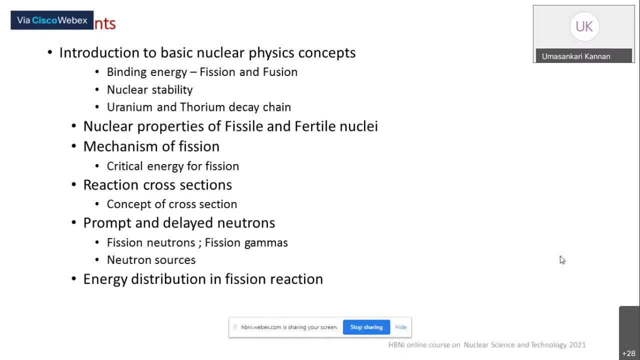 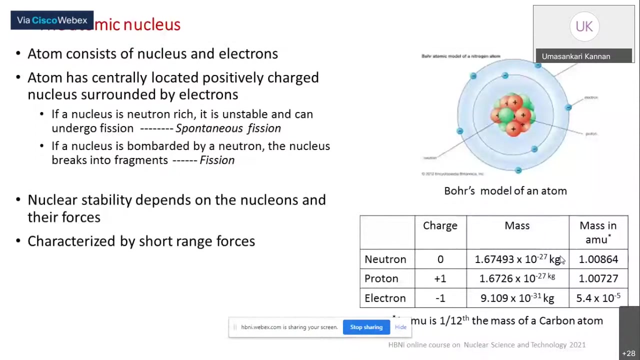 or delayed neutrons. and what are the neutrons and what is the fission reaction? They are all centrally placed, charged, and the electrons are orbiting around the nucleus. If a nucleus is neutron-rich, it is unbiased, It is unstable and it can undergo fission. 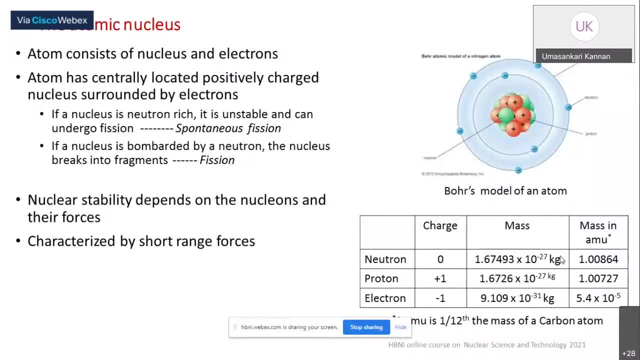 So this process is called as a spontaneous fission. But if a nucleus is bombarded by a neutron, the neutron the nucleus breaks, makes small fragments, activity, stability for neurons and forces. You know that a nucleus is characterized by the neutron and proton. 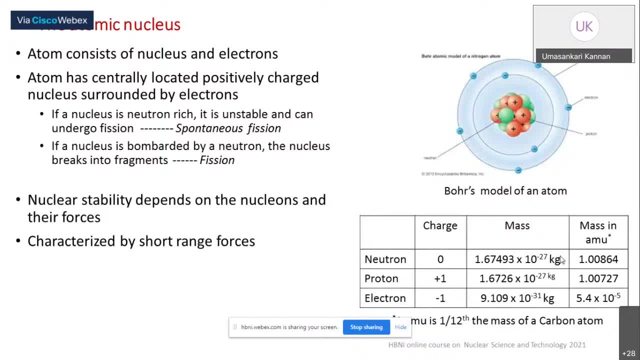 Neutron is massless. Neutron is massless, Power is charge-less and proton is positively charged. And here I have given you the mass of a neutron and mass of a proton in terms of AMU, And the electron is about 1,861 times lower than that of electron mass. 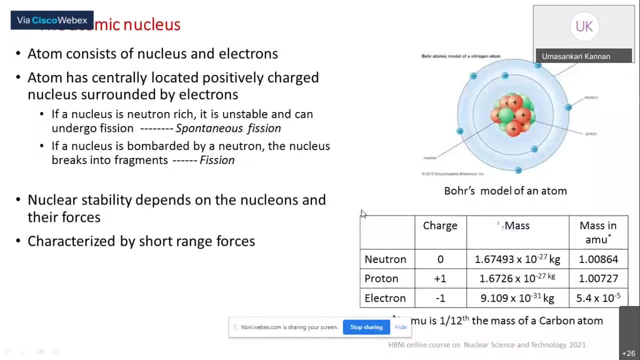 1,861.. to the massive carbon atom. Now, What happens in a nucleus? Nucleons are present inside the nucleus and they are characterized by the short-range forces. A neutron can get converted into a proton or into a neutron. 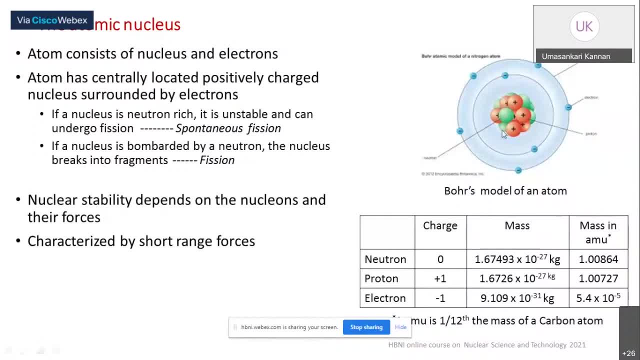 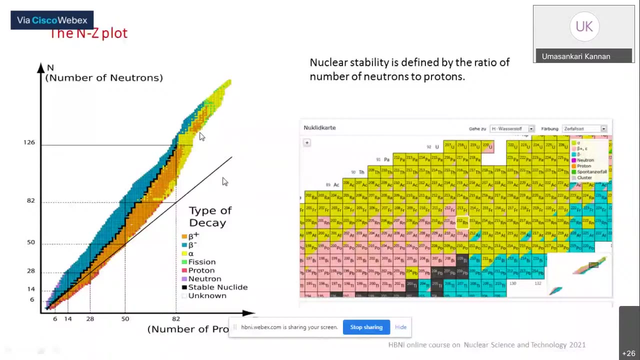 All these processes are happening inside the nucleus And that's where they're all. in terms for nuclear physics, It's called as nucleons and they are characterized by short-range forces. The whole process is that it declares stability line, where we call this as NZ plot. 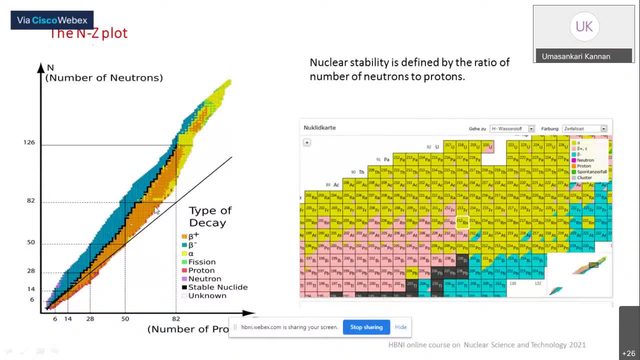 These are neutrons and number of neutrons. It usually follows this black dot, black curve And on the left-hand side you have the beta minus decay. On the right-hand side you have the beta plus decay. There are so many elements in the periodic table. 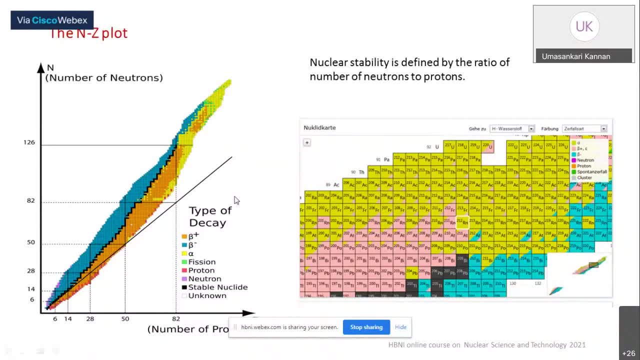 Which are because of these radioactive. So the stability is dictated by N and Z. It is defined by the ratio of the number of protons to the neutrons. So that is why it is important to see why certain elements are becoming radioactive. By emitting a beta, they become more stable. 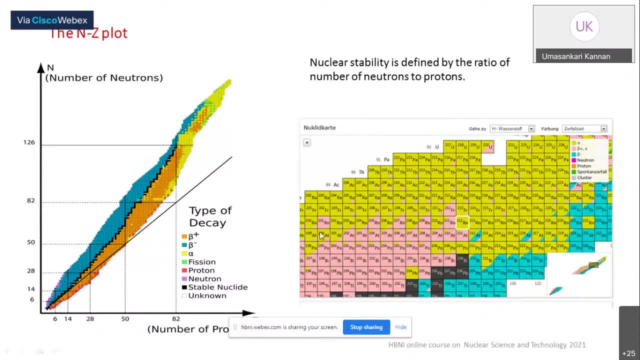 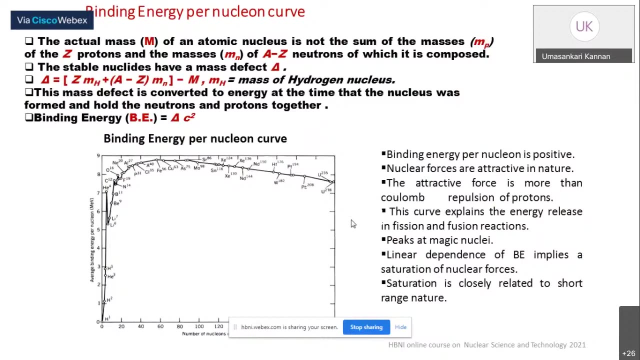 Or by emitting an alpha, they become more stable, And why some of them are stable by nature, And some of the numbers also, you would be knowing. This brings us to the topic of binding energy, Not just some of the masses of the neutrons and protons. 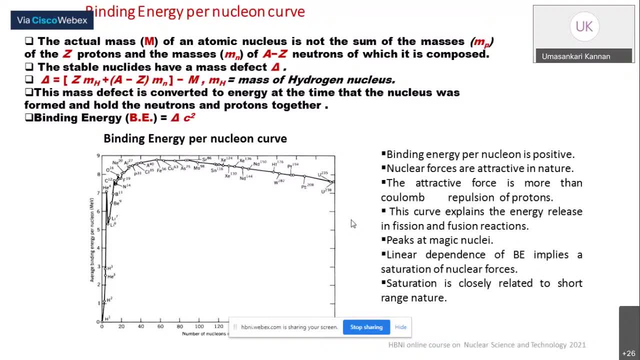 So there is something called as a mass defect. This mass defect is energy, And that is what is binding the nucleus. So this mass defect is termed here as number of protons into mass of protons, The number of neutrons, which is A minus Z. 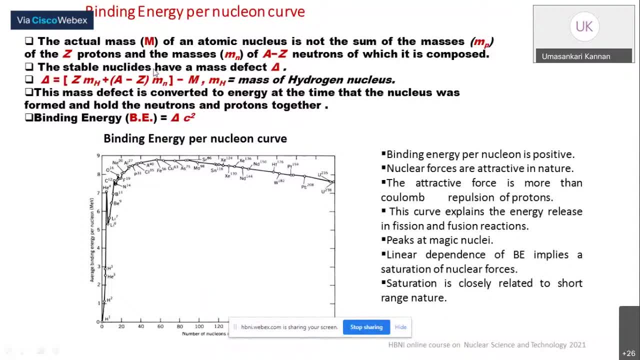 Minus mass of neutrons. So this is called as defect. This is called as a mass defect. The energy and the equation of the principles, This delta times square, would be the binding energy of the nucleus. Here I have shown you the binding energy of the nucleus as a function of atomic number. 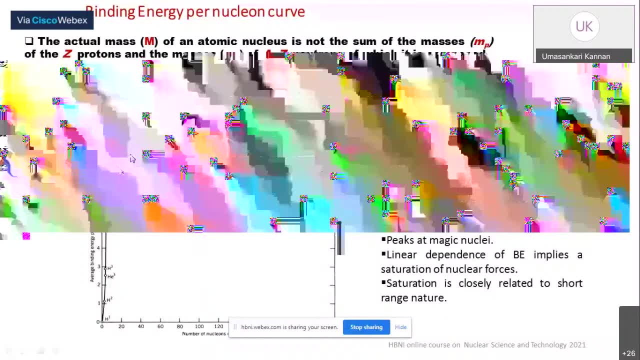 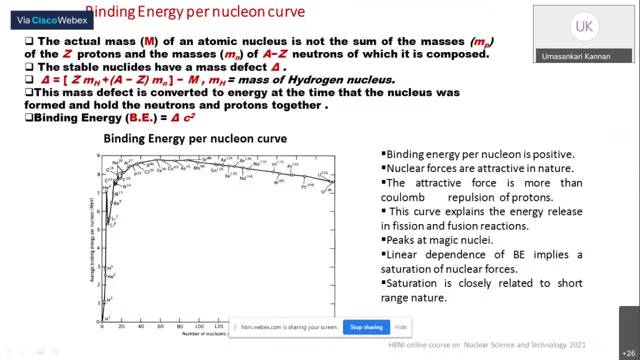 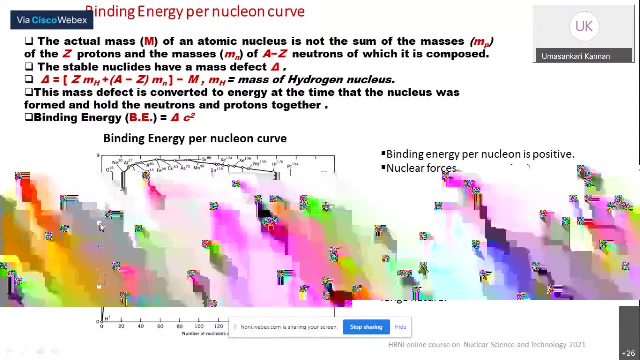 And here you can see there are some sharp peaks which are basically the stable nuclei. This, in the y-axis, is called as the binding energy. So this is the binding energy. Now you can see that around this number. So this is the binding energy. 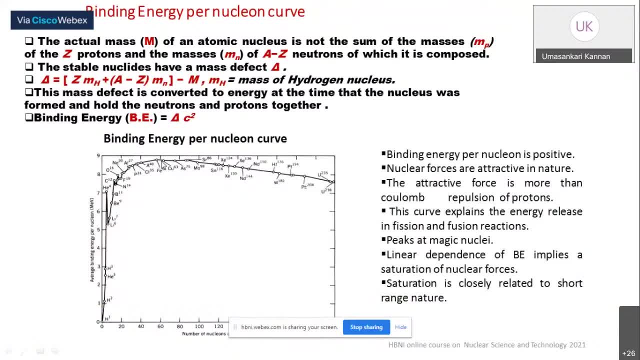 And the one thing that you are having at this table is the ion 56. And here you can find that uranium-235 is somewhere here around 235 mass number. So you would see that why fission is happening or why fusion is happening. 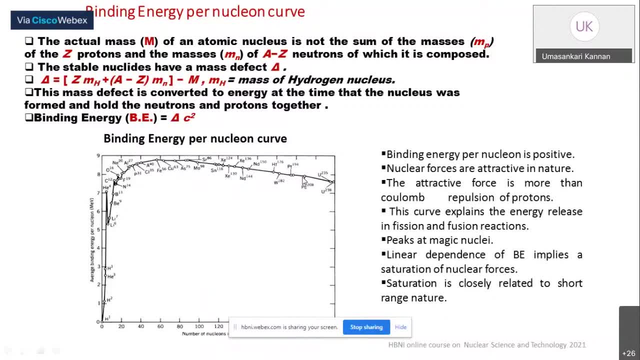 Uranium-235 nucleus when it neutron to 36 and it becomes unstable. and it become, and it splits into two efficient products- higher binding energy. thereby it releases the energy equivalent to the difference and its efficient products. so the binding energy per nucleon is always positive and the nuclear 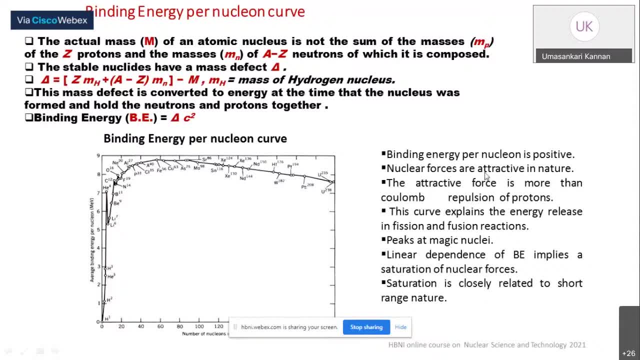 forces. you know by now. i have already explained to you that it is attractive by nature. so the attractive forces is more than the coulomb repulsion of the protons, and so this is the curve which explains why fission is releasing energy, or in other words, fusion two light atoms. 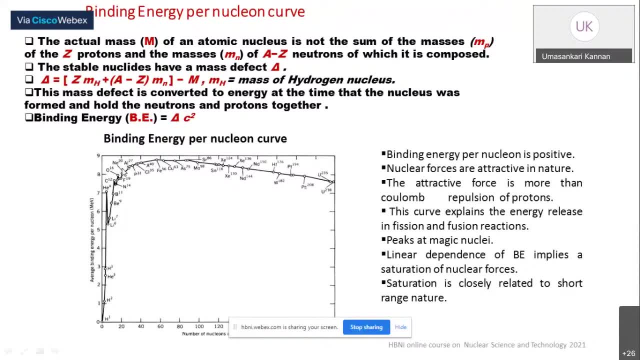 can fuse also and give you the energy to become more stable. and then who speaks? and then there it's very difficult nuclear. so these are magically. the linear difference of binding energy implies a saturation of the nuclear forces, so this saturation is closely related to the short range. 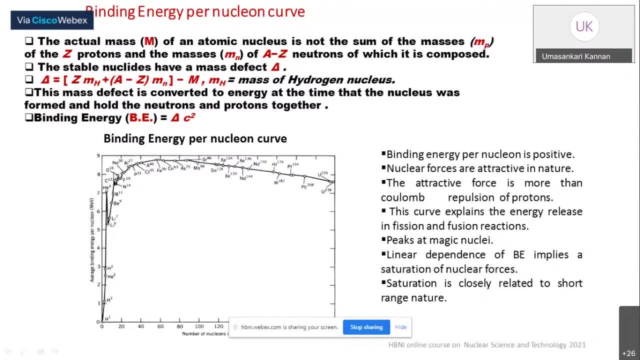 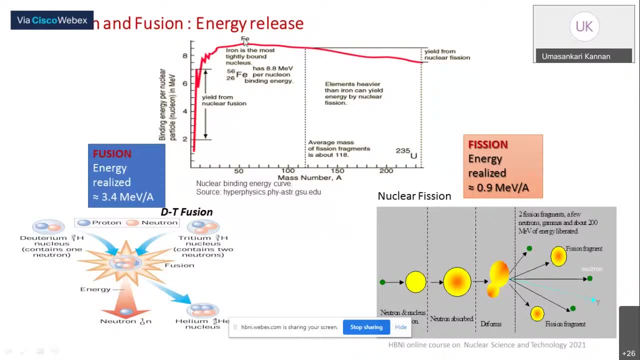 forces. so if you have clear, i have got clarity about this binding energy. you know that. why fission or fission, energy is going to be or energy is going to be released in fission. so here you can see i have right, a little more enes of this. so this difference is what is going to come out as efficient. you know, elements heavier than ions can yield energy by nuclear fission. here, if at lower mass numbers- this is a fusion, dT, fusion dC and C, which energy is realises at about 3.4m3 per nucleon Ne. тогда n spokesman keteper. 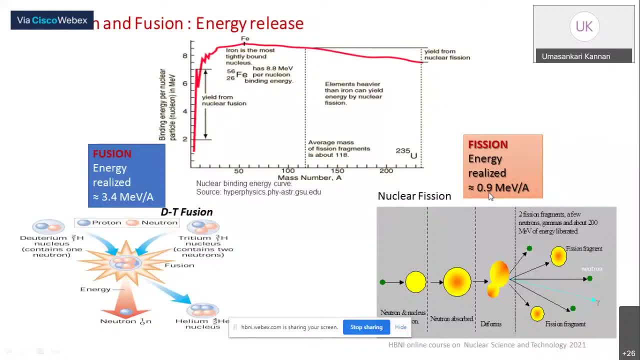 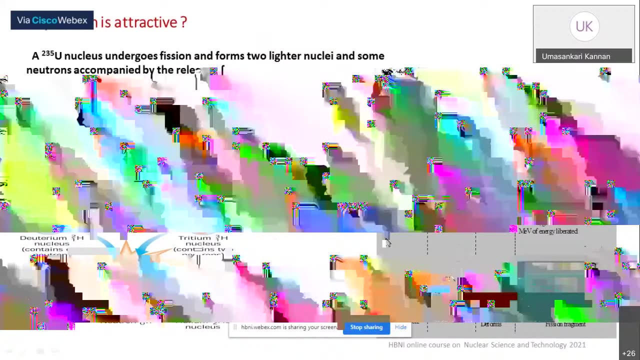 And whereas in fission it is about 0.9 MeV per nucleon. So that is why it is 0.9 MeV per nucleon and mMeV of energy is released in a single fission. Okay, So now we have got the idea of binding and energy. 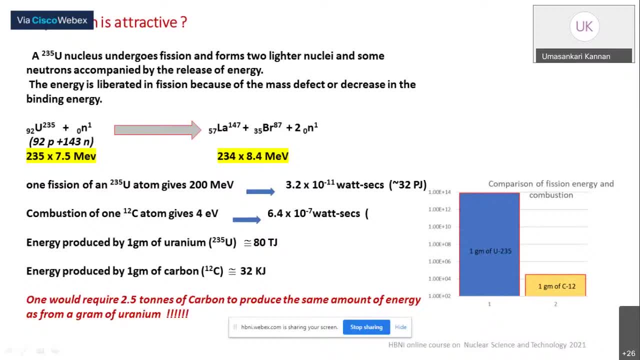 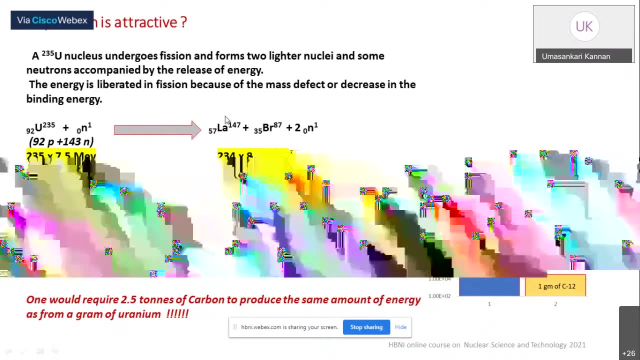 Now let us see why fission is attractive. I have already told you that a uranium-235 nucleus undergoes fission, forms two lighter nuclei. Let us take an example: When uranium-235 nucleus absorbs a neutron, it becomes. It has two fission products. 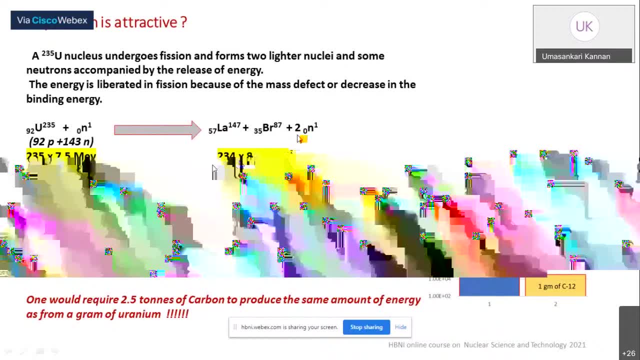 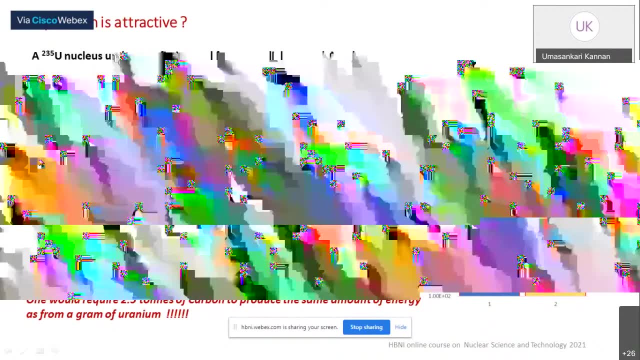 On the right-hand side we have 34 neutrons. Average binding and energy per nucleon is about 8.4.. Whereas on the left-hand side we have 235 nucleons And the average binding energy is 7.5 MeV. So this results in a difference of about 0.9 MeV, which gives around 200 MeV of energy. So one fission of one atom of uranium-235 gives 200 MeV of energy, Which, when you calculate in joules. 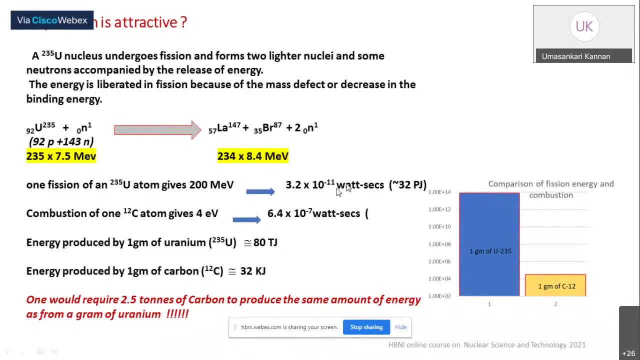 It turns out to be 3.2 joules per hour Minus 11 watt-seconds, or around 32 picot-joules. Now just compare this with a combustion of one atom of carbon. One atom of carbon gives an energy of about 4 eV on combustion. 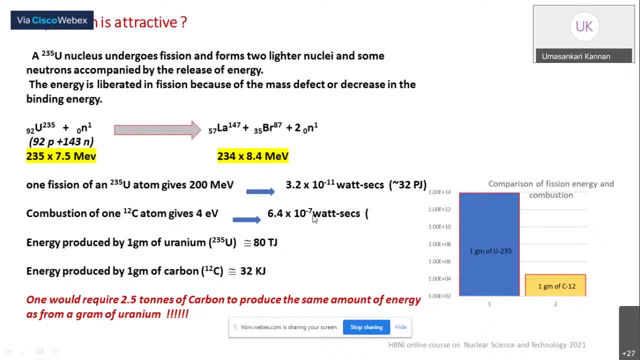 And this gives 6.4 into 10, to the power of minus 7 watt-seconds. Or it gives you: If you look at the energy produced from one gram of uranium, you do the mathematics, you will get 80 terajoules. 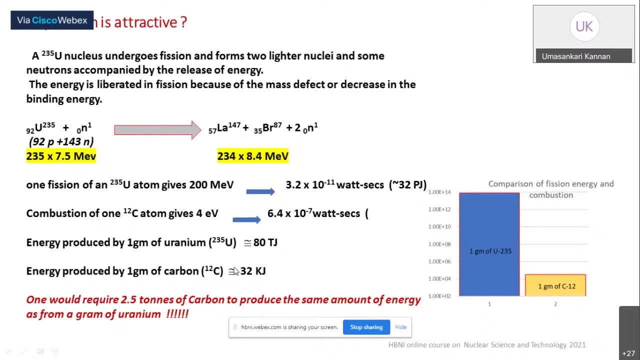 Well, whereas the energy produced from one gram of carbon is about 2.5 terajoules, Or in other words- I have done statistics- it shows that you would require about 2.5 tons of carbon to produce the same amount of energy from a gram of uranium. 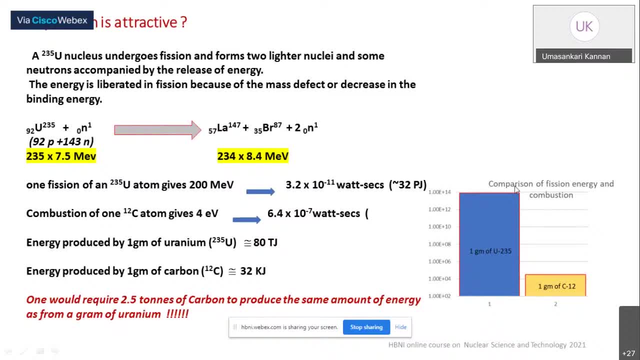 I have tried to pictorially show this. This is a log scale in y-axis And you can see this: one gram of uranium equivalent is giving you so much of energy, whereas one gram of carbon is giving you this much of energy. So that is why we are in business. So that is why fission is attractive And you will be able to do it. So that is why fission is attractive And you will be able to do it. So that is why fission is attractive And you will be able to do it. 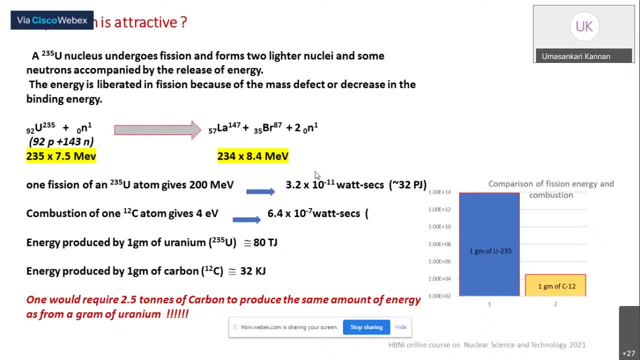 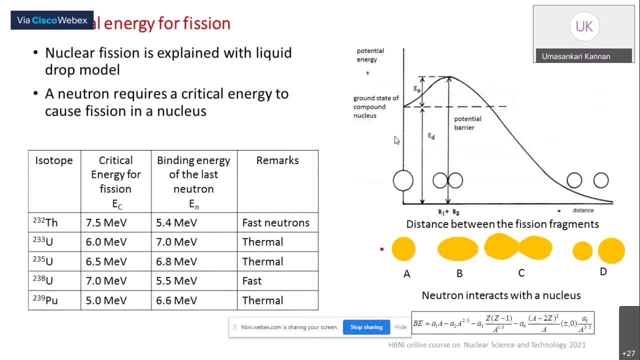 And you will be able to do it. And you will be able to do it. Let us talk about fission. So how to explain the nuclear fission? Generally, we have used the liquid rock model to explain nuclear fission. The nucleus is assumed to be drop of a liquid. 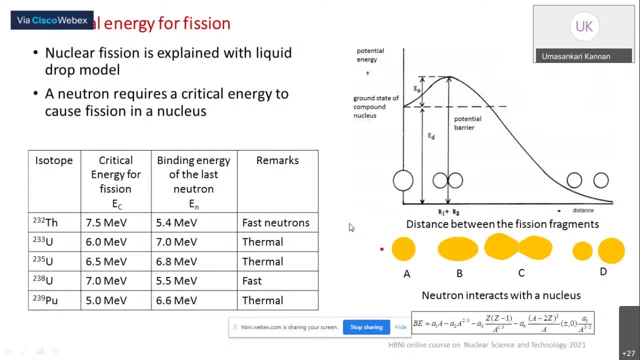 So a neutron requires some critical energy to cause fission. in a nucleus. say, a neutron is absorbed by a nucleus and it is somewhere here the ground state of the compound nucleus, and because here the energy is such that it will be able to break this rock to. 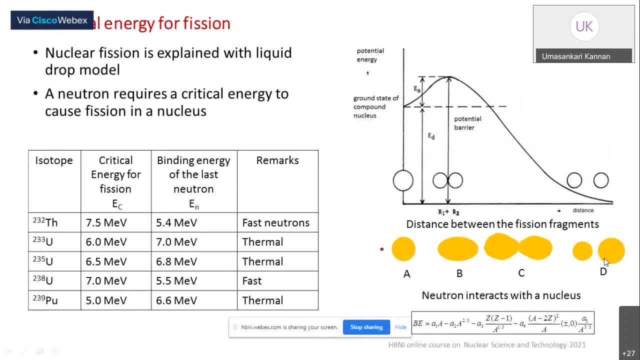 imagine a surface tension of the rock which is required by the neutron to break the nucleus, or this is called as a critical energy of the nucleus for the neutron, and here, finally, we get two products. and these are the different stages by which the fission process takes place. now here you can see that. 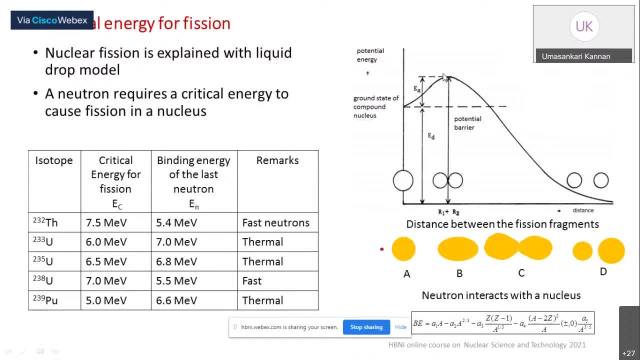 the uh, for example, the critical energy is about 7.5 mev and the binding energy of the last neutron is 5.4 mev. so this is not enough to cause fission. so you have to have a fast neutron to cause fission. 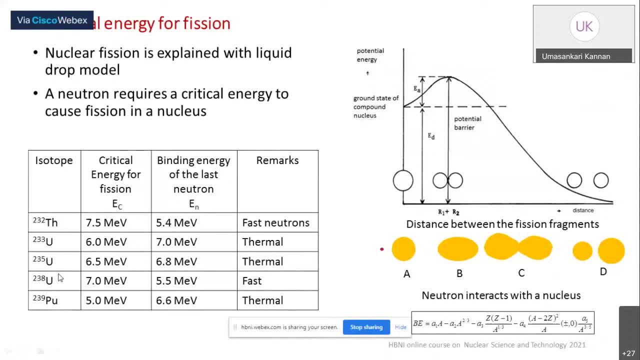 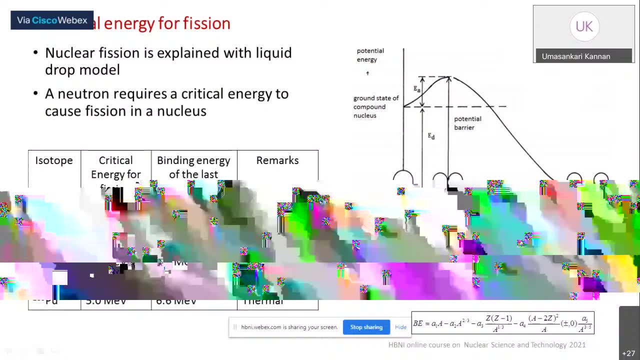 in thorium-232, whereas look at uranium-235. the critical energy which is required, which is difference, is about 6.5 mv, and the binding energy of the added last neutron would be six point ninety three summon system, which means that 7.5 mv, Ori, 6mb, and now here even, 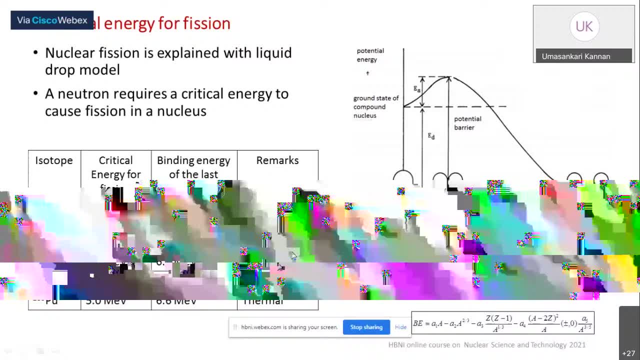 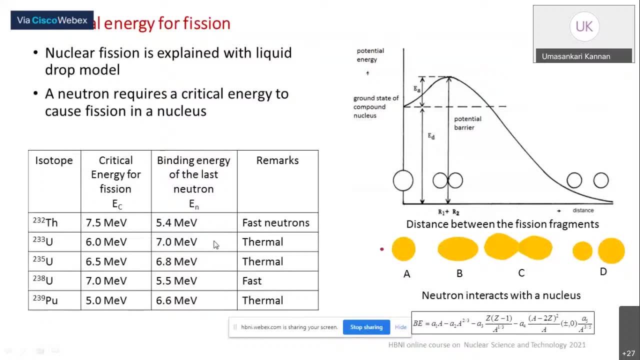 the total at 2.5, 10 to the dock. so it's like uranium to the one to the top. so and or one, our brown natural energy, which is seven empire, is equal to zero and we have got to be up. no, and you take the aura, and when you take the aura, you 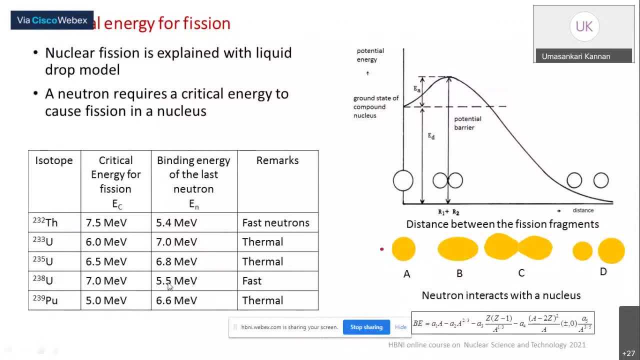 againики, this is rightертвants and this is the root area of the human iron, even if you take even, is a critical energy for fission and the binding. So, by assuming that the fission process using the liquid of the nuclear we can, which is required to cause this fission, 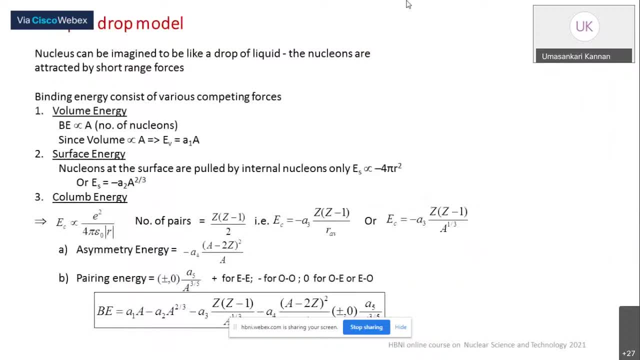 A little more about the binding energy and the liquid drop model. There are so many terms and this is how it defines the binding energy of the nucleus, The volume energy term, which is shared volumes of, and so it is proportionate by r square, or it is proportionate by r square or it is proportionate. 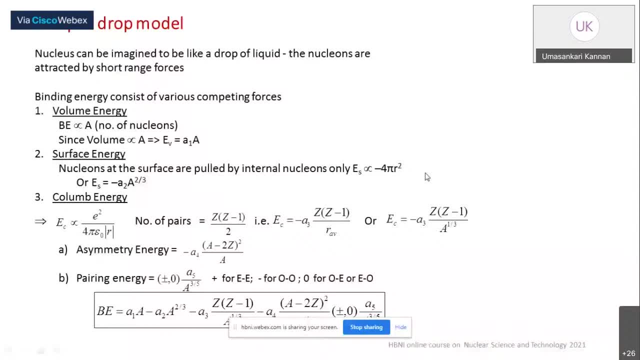 by a, to the power of two by three. then there is a coulomb energy which is the number of pairs, different atomic number. So this is another term which is giving the coulomb energy and there is an asymmetry part, KBT, in the pairing part. So all these terms put together, 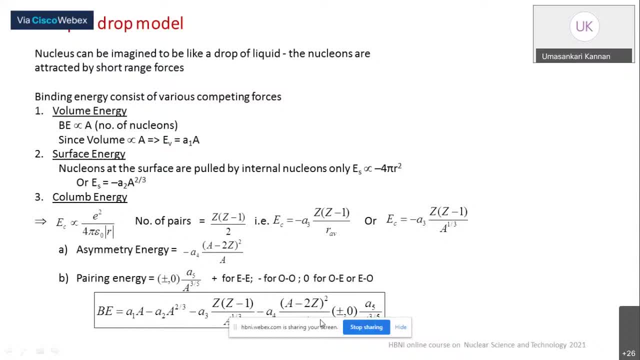 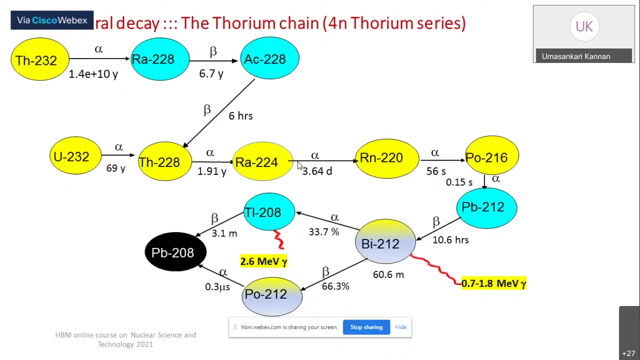 you get the finalnamenebing in a nucleus. So this n ter이지 of a pervasion nuclear part, Wednesday 0430.. either a fission or a fusion. talking more about told you that some of the elements are either beta emitters or alpha emitters. so here i have tried to. 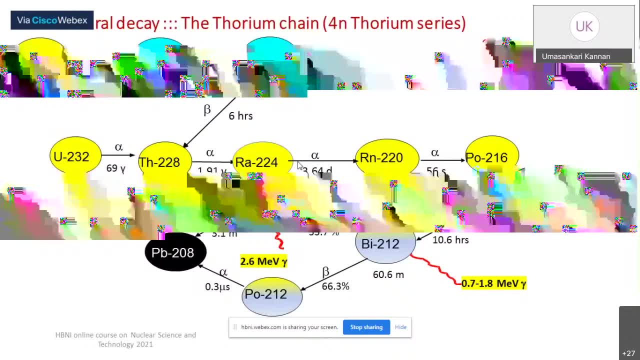 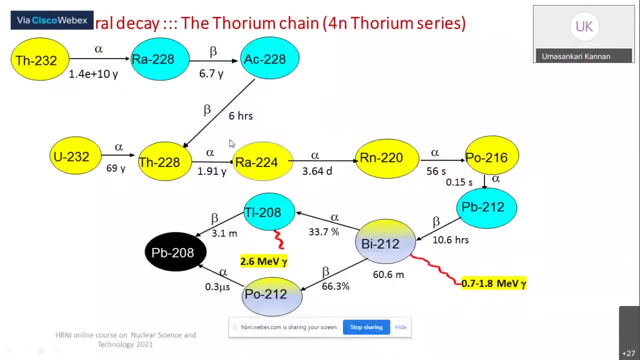 give you a natural decay of thorium nucleus. most of these are alpha emitters, some of these in between you can see the beta emitters and that actinium. so a thorium fuel can be characterized by this gamma emitter, which is the natural process in the decay of the thorium isotope, and so that is why it is very it's. 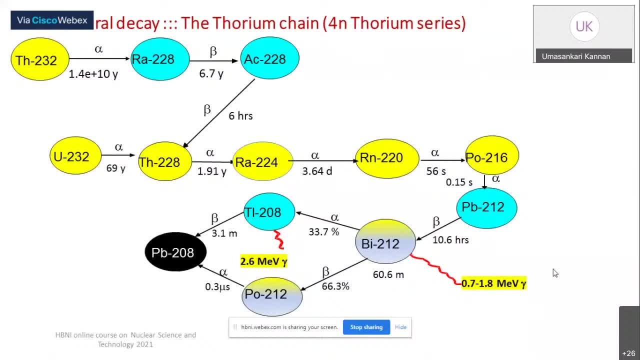 proliferation resins, fuel will come as much. these are all emitters and you can see thorium has a half life of about one 10 to the years. see this. uranium-232 is a manifest idea of, if you look at this, awak or opium. 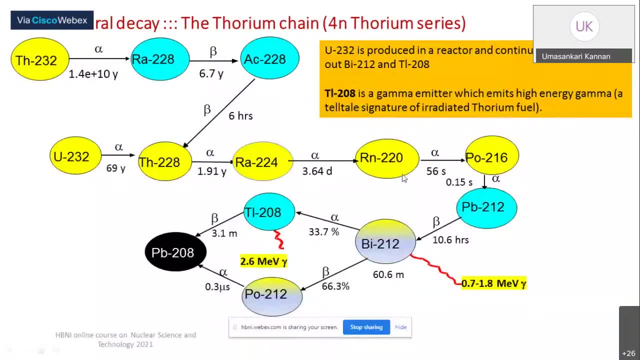 it takes 10 years to die is taking 10 years. every 10 years you need to defeat thorium, which can give you Baron tiesick, but later the whole thing will be with ktum 3, with chrompetum is produced in the reactor also and it continues to decay, giving out. 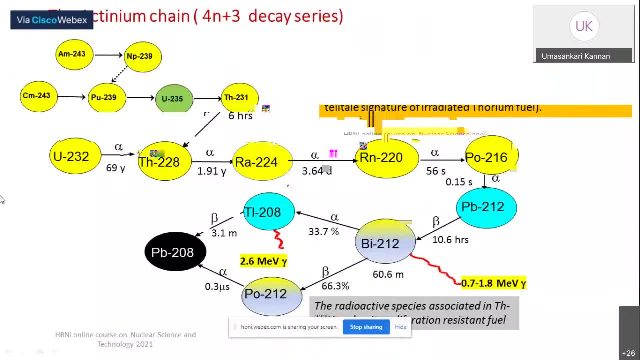 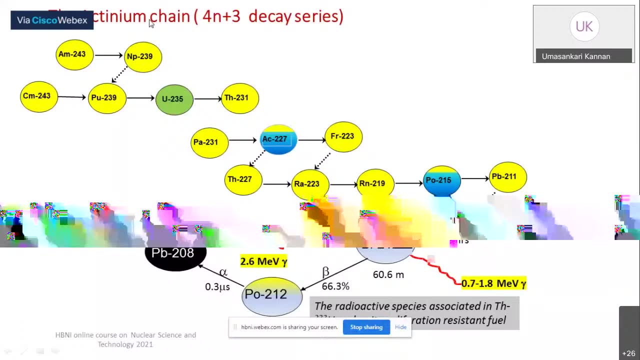 this bismuth, and and that is why, when i am using thorium fuel in a reactor, it is this uranium corrector. Now let us talk about a uranium decay chain In the uranium. here you can see that uranium-235 is an alpha decay product of plutonium-239.. 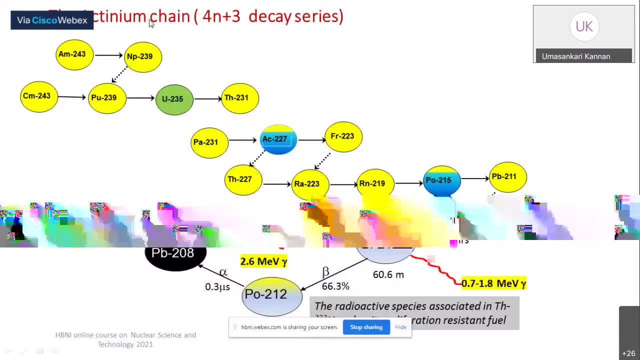 Plutonium-239,. these are all, of course, not found. Ameritium-243, again, these are all produced only in the reactor. But here you can see, naturally uranium-235 is an alpha decay product. Plutonium-239 gives you plutonium-239, and there are other products which are found in the decay chain of uranium-235. 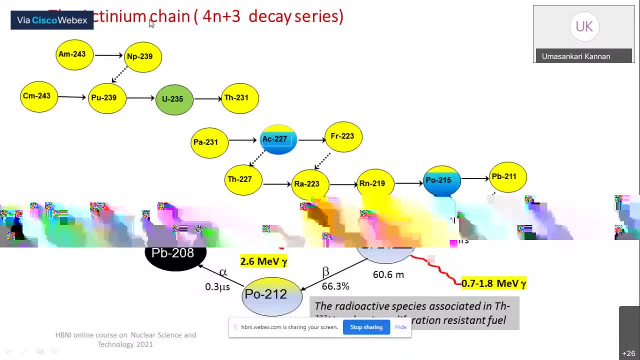 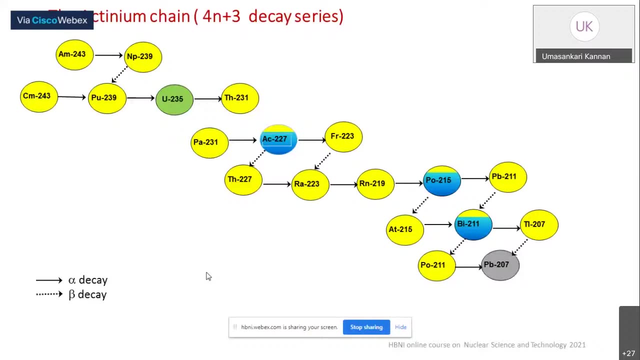 So these alpha decays are characterized by the straight lines here, and the beta decays are characterized by the dotted lines here, And finally you get a stable product like lead in the decay chain. But all these are what I wanted to impress upon you- is, apart from being radioactive emitters, 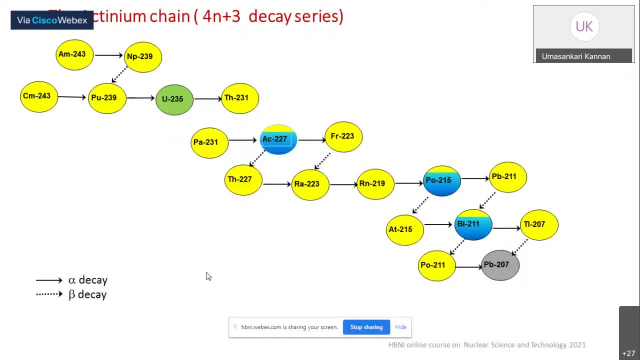 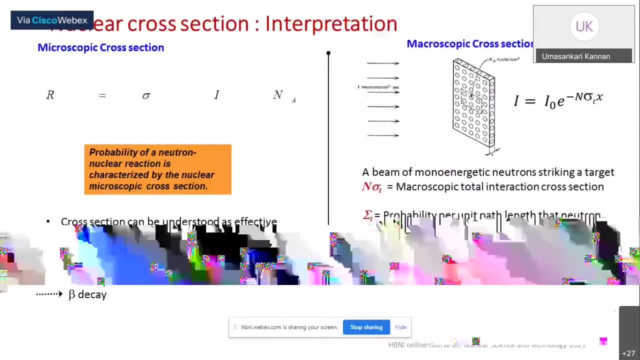 natural decay will happen. This is a type of nuclei for the isotope. Now let us talk a little about what exactly is going to be done in fission process. Okay, we know fission process is taking place, but there is something which is important is the cross-section for any particular reaction. 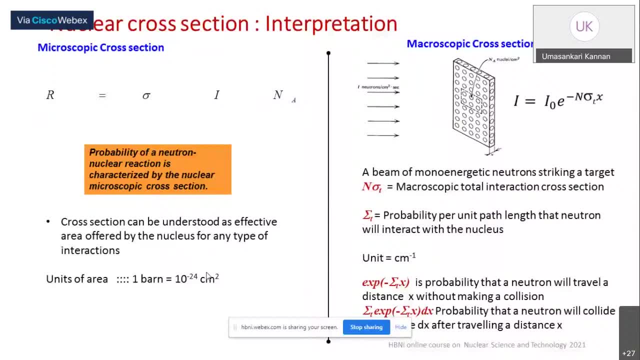 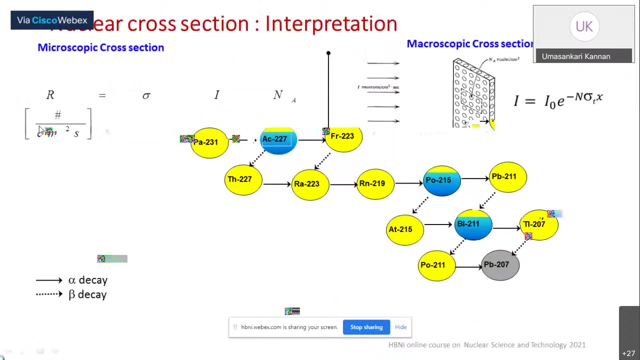 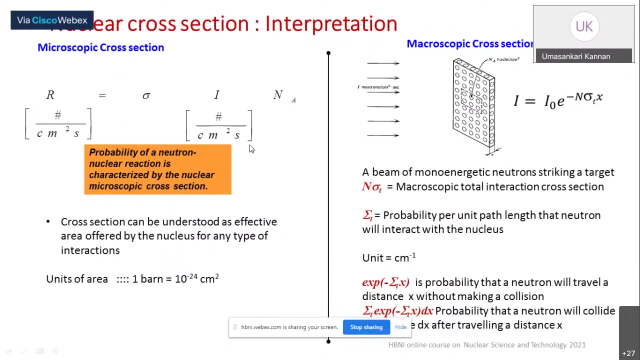 Let us talk about a nuclear cross-section. Let us try to find out the interpretation. What is the cross-section? See, you all understand about reaction rate. Reaction rate is nothing but the cross-section multiplied by the number of interactions. So here, if R is the reaction rate, which is the interaction rate, I is the intensity of the neutrons. 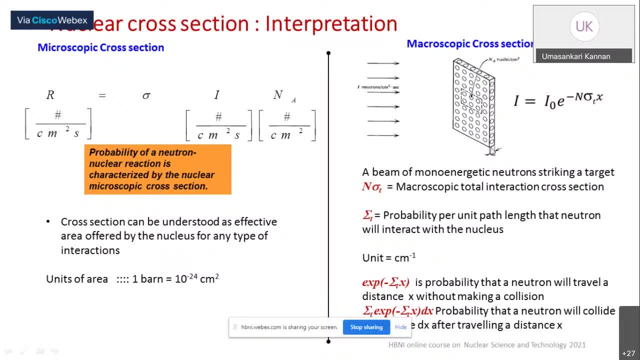 and N is the number of the nuclei in the target here. Now. this reaction rate is proportional to the intensity and multiplied by the nuclear by a constant. This constant is called, as a probability, of a neutral on real interaction and it is characterized by the microscopic cross section. This sigma is what 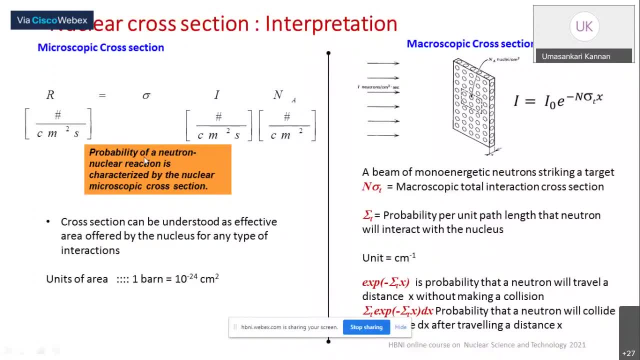 is very, very important. It is called as a cross section for any particular type of reaction and it can be seen as a probability or effective area offered by a nucleus or a typical type of reaction. Since this area is very, very small, we talk in terms of Fermi distances, which is the 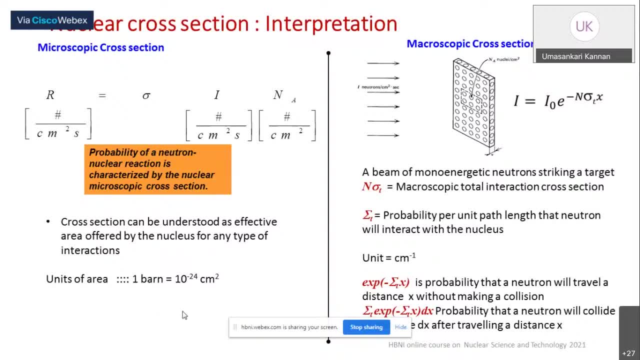 size of the nucleus, So the units of area also has to be very, very small. So the unit is one band which is 10 to the power of minus 24 centimeter square. This is a microscopic cross section. This is the property of a nucleus for a nuclear energy. So 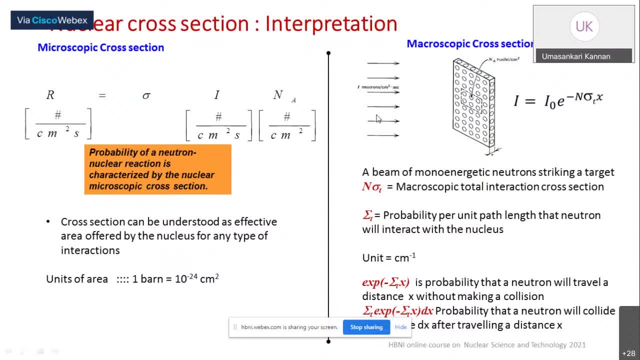 they have different energies. I will come to all that a little later. Now this is the microscopic cross section. We have another microscopic cross section. You consider a sample which is placed here, a beam of neutrons which is incident perpendicularly on the sample, and how much. 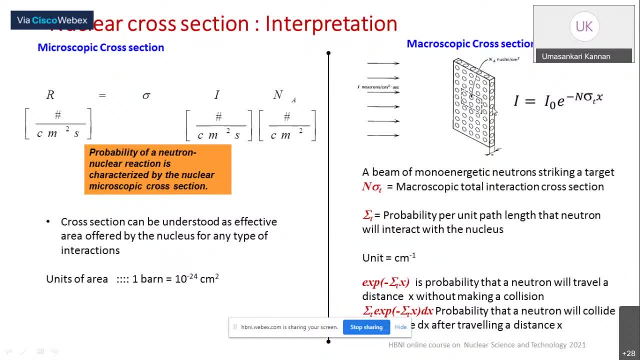 interaction takes place in the sample and what is the net intensity of neutrons, Neutrons, which is coming out of the sample, which is given by this? I is equal to. I naught into e to the power of minus n, sigma t x. x is the thickness of the sample, n into sigma t is the 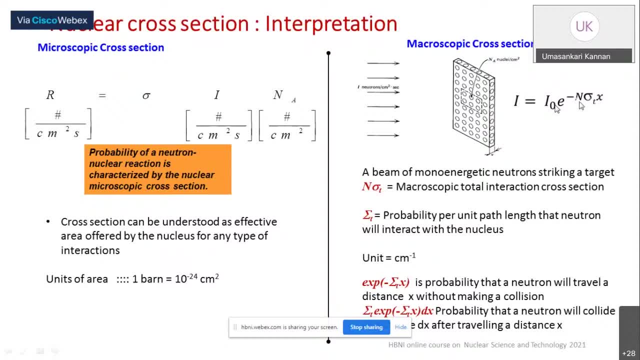 total cross section of this particular target and n into sigma is the macroscope total interaction cross section, So a beam of mono energetic neutrons which are striking the target. this n into sigma is called as a total probability of this particular target, And so the sigma t is called as the total probability And this is the probability. 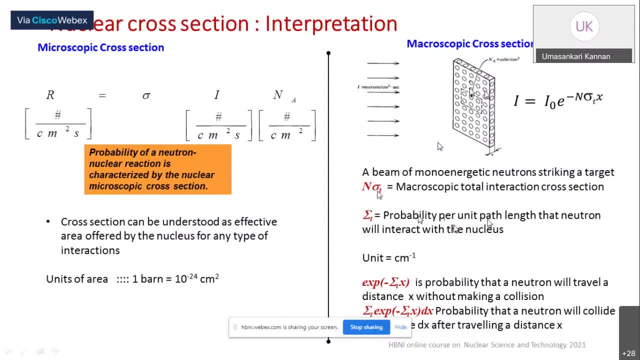 per unit length. All this is x. here The neutron will interact with the nucleus, So this, if you take this unit, will be centimeter inverse. Now we will talk about this quantity, which is e to the power of minus sigma t into x. 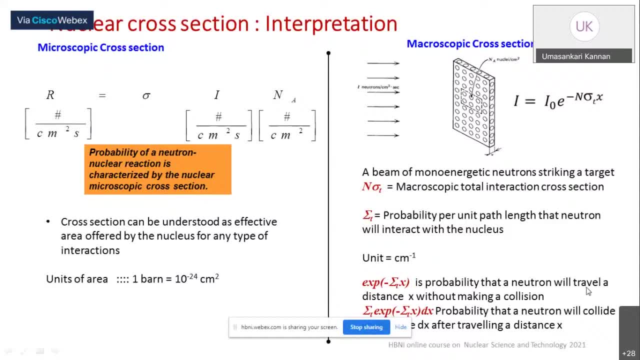 D, x, x is equal to sigma t Right here. so the mass resistance is: is is equal. Now, what should be given from this? I just have From this left line, So from the left forces, descent time, Same 얘기를, Yes. from this right line. And now, what should be given by this independent camera? well, there is no difference between, for example, the left halftone of the laser light beam side and first light gradient. But we do not want to sketch this. So when we see the volumetric 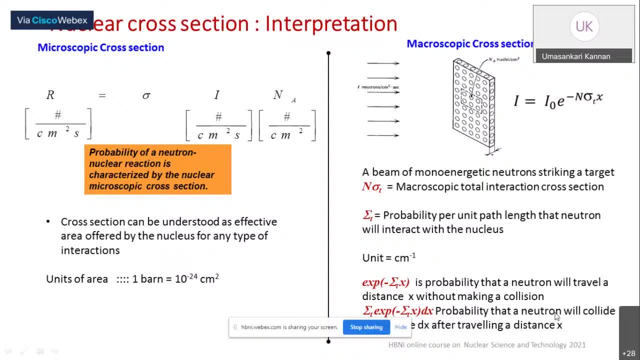 So this is the kind of the interaction probability which has happened with a mono energetic neutrons which is crossed, which is hitting a target and it is causing interaction in this particular sample for target. So this is basically the microscopic cross-section or probability of a neutron-nuclear interaction. 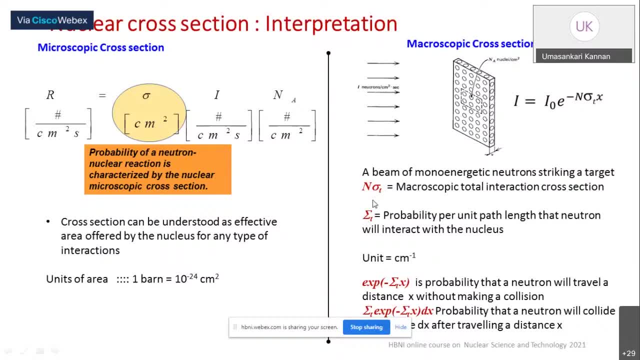 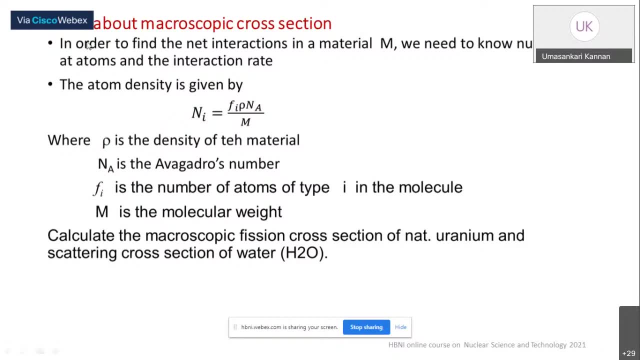 and this sigma is called as the macroscopic cross-section or the total nucleides in the sample or particular target. There is something more about this microscopic cross-sections. In order to find out the net interactions in a material, M, we need to know the number. 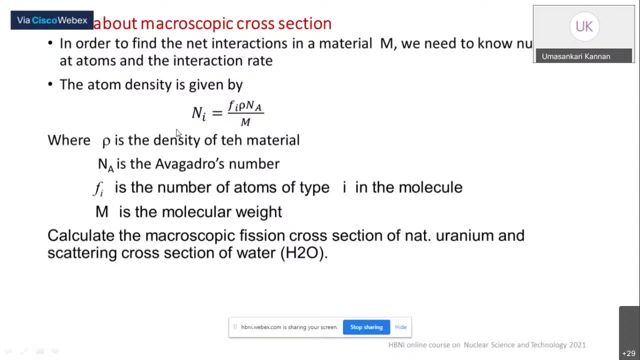 of atoms and the interaction rate. Okay, So this atom density of any particular target is given by, you know, the Avogadro's number, rho, and rho is the density of the sample and m is the molecular weight of the sample and fi is the fraction of atoms of that particular type in a molecule. 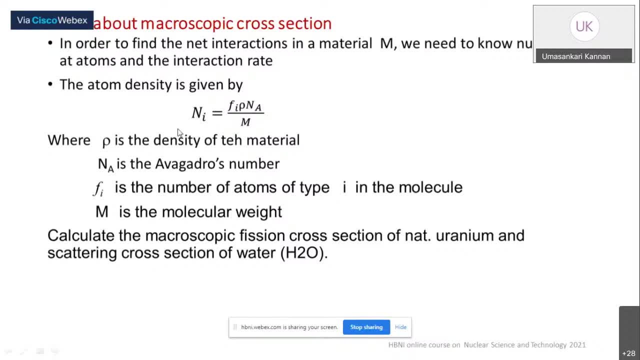 So this is the total atom density of a in a sample which is given by ni is equal to rho na by m into fi. So now this ni will be the number of muons, This is the number of nucleates in a particular sample, and if this is multiplied by the microscopic 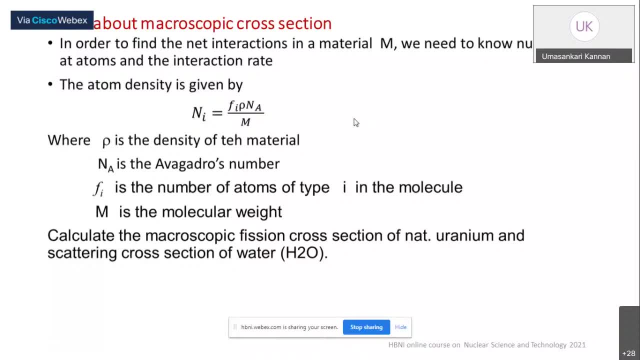 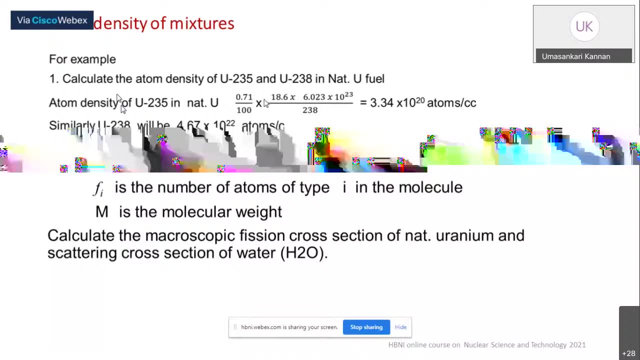 cross-section we would get the macroscopic interaction cross-section Assignments also, in which you can get the atom density. but here I am trying to impress upon you what would be the atom density of uranium-235 or uranium-238 in a natural uranium. 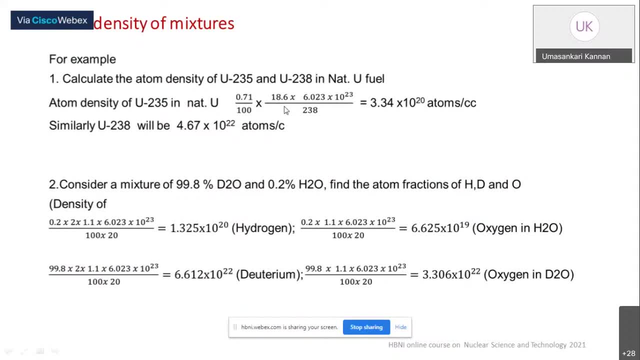 fuel and how to go about it: 18.5.. So 18.6 is the density of uranium-235, uranium, natural uranium, and this is the Avogadro's number. this is the molecular weight and this is the weight fraction of uranium-235. 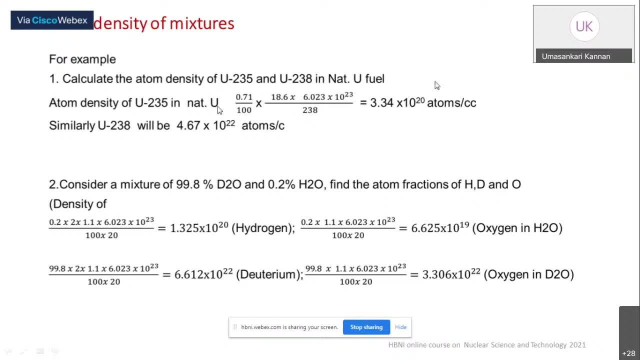 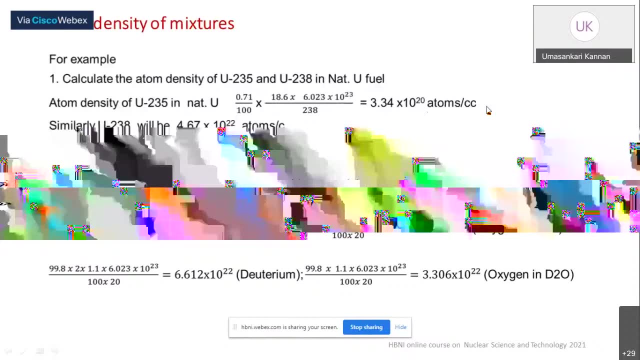 in natural uranium, which is 0.7 percent, and so we get around 3.3 into 10.. You know, for natural uranium in a sample. Similarly, the uranium-238 would be 467 into 10, to the power of 22.. 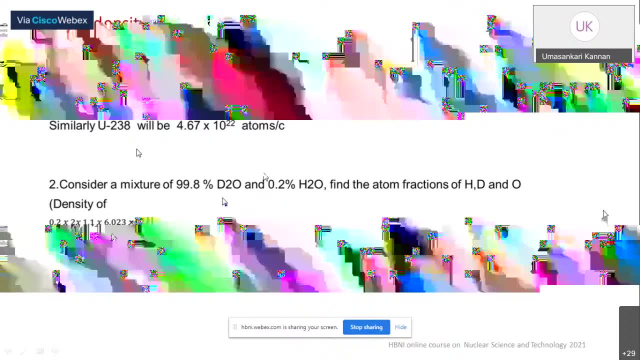 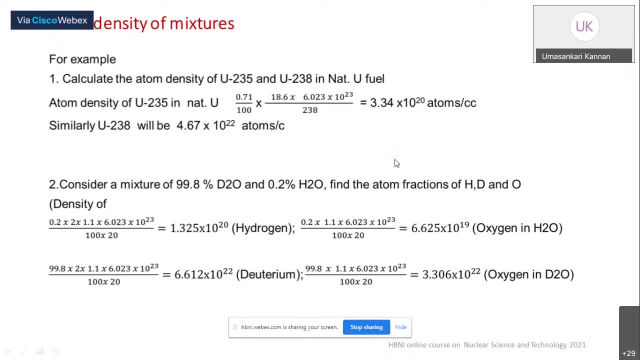 Similarly you can calculate for a macroscopic interaction. You can calculate for a mixture of light water and heavy water. Here I have taken an example of light water as 0.2 percent in heavy water of 99.8 and how I have found out the atom fractions. 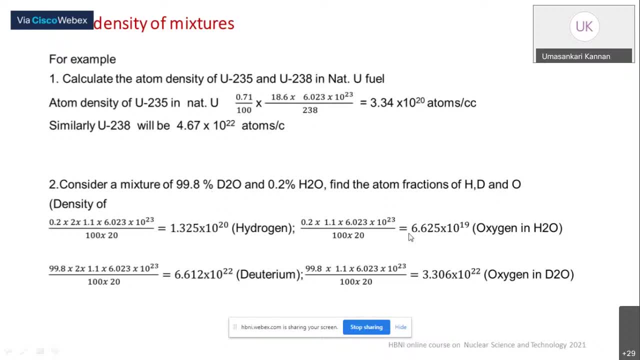 I can leave this presentation with you so that you can see all these later. but basically you can calculate the number density of each and every component of the fuel or the coolant or the modulator which is being used. So this is the number density of each and every component of the fuel or the coolant. 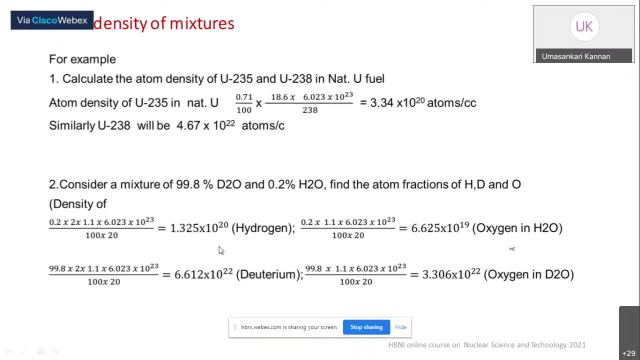 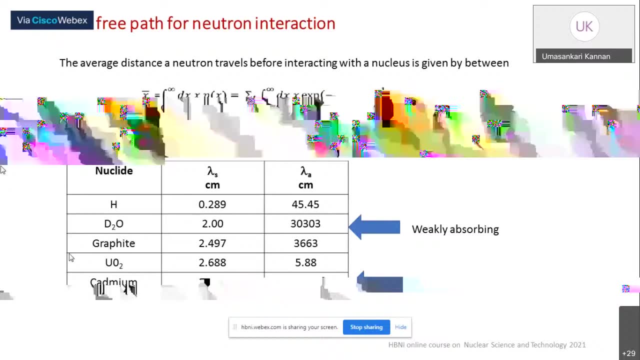 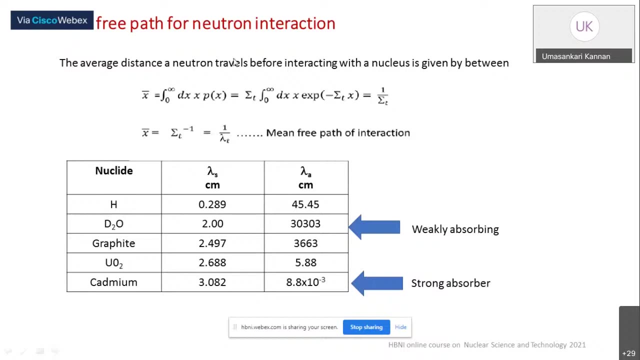 or the modulator. So here, in this case, it is oxygen or hydrogen or deuterium. You can calculate the atom density for each and every mixture. Now I was telling you about interaction. Now, this interaction is also. what is more important is the. what is the mean free path. 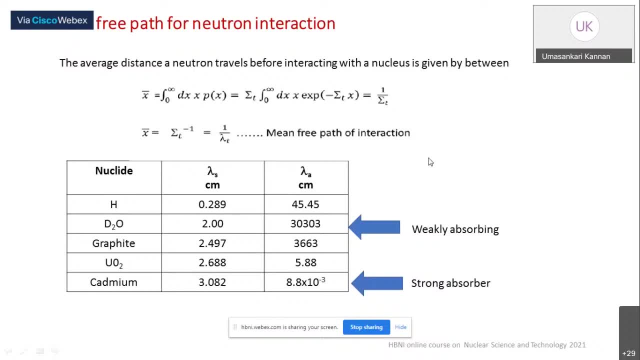 for interaction. I was telling you that it is collided and uncollided. It is. What is the? what is the interaction rate? Now, if I talk about a probability of interaction, I can define an average distance, which is a neutron can travel before interacting with the nucleus is given by, let us say, x, bar. 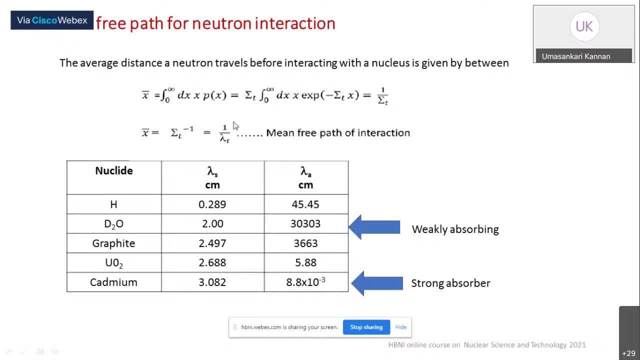 The probability of P of x, x, dx. if I integrate it from 0 to infinity, I can this. I can reduce it to sigma t into dx x, exponential e to the power of minus sigma t x. So this is the probability of P of x. 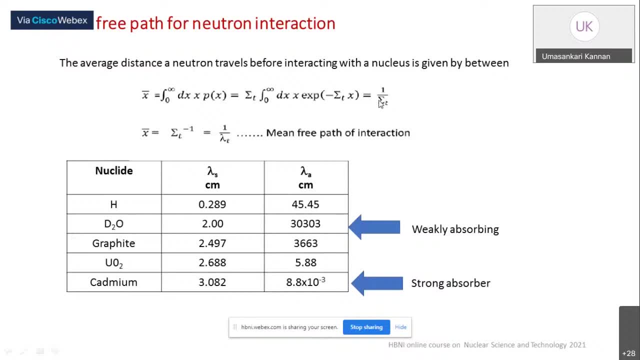 So this is the probability of P of x. So this is nothing but one by sigma t. Sigma t is the total cross-section interaction And this total cross-section, one by sigma t, can be as thought of as a mean free path. 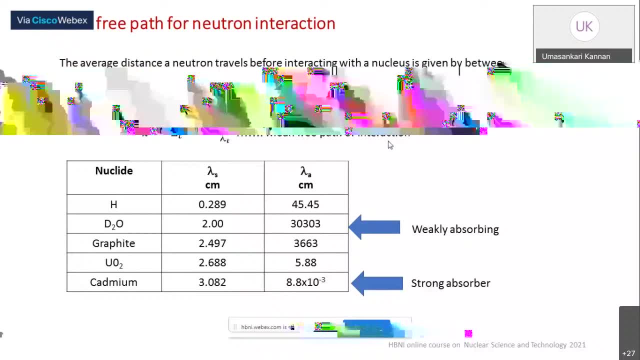 of interaction. See, that is a neutron traveling in a sample, a beam of neutron traveling in a sample, And what happens is that it is what is the mean free path or mean distance over which over which this interaction can take place, For example, if it is a very strongly absorbing medium. 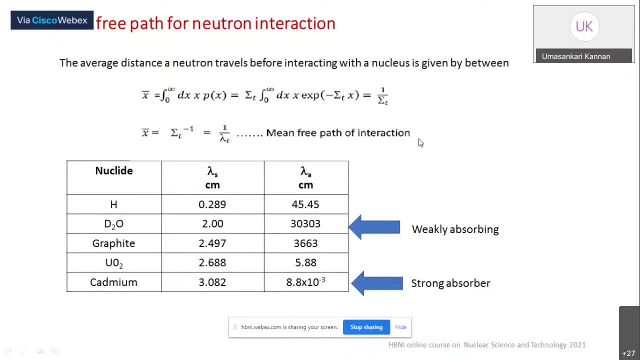 it is a very strong medium. and if it is a very strong medium, it is a very strong medium. And if you consider it for D2O, the scattering mean free path is 2 centimeters, whereas the absorption mean free path is 30,000 centimeters, which means it is a very, very, very weakly. 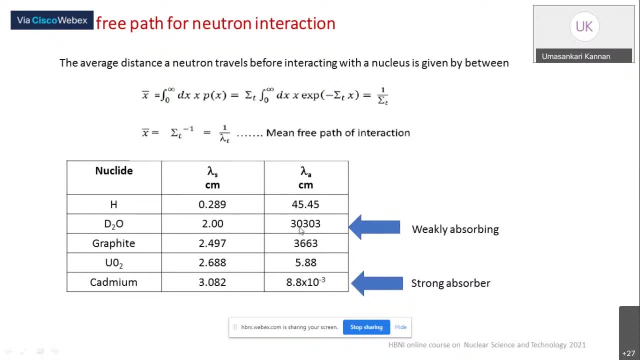 absorbing medium, And that is why we use heavy water in the thermal reactors as a medium. In graphite, again you can see that the absorption mean free path is 30,000 centimeters In peroxide, which is used as a neutron absorber for thermal neutrons. here you can see that. 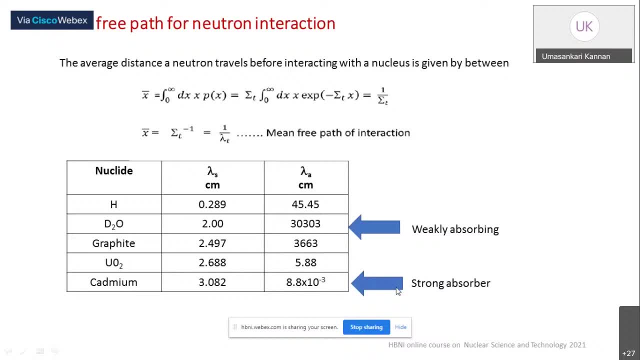 the mean free path for absorption is very small. That means it is a very, very strong absorber. What I want to impress upon you here is that what the nuclei will interact with neutrons in different ways, And so that is why these cross-sections are important, and that is why we have to 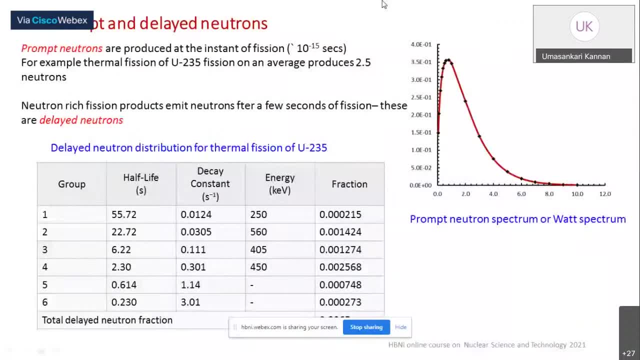 be free. Now let us talk something more about the neutrons. You know, in a fission reaction, neutron is getting absorbed, a compound nucleus is formed. the compound nucleus splits into two fission products and also produces some neutrons. 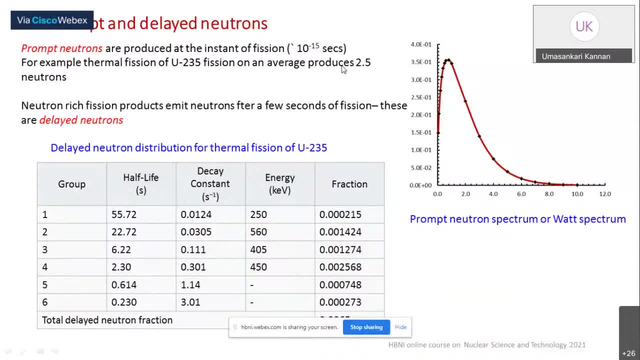 Now there are different types of neutrons which are being produced. The neutrons which are being produced at the instant of fission is called as a prompt neutron, For instance, the fission of 2.5 neutrons. you have a study textbooks: 2.5 neutrons are 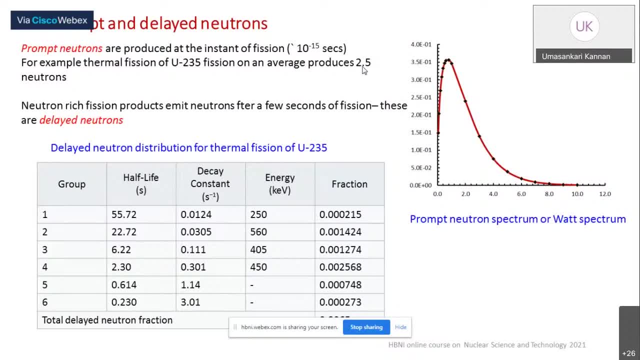 produced in every fission. But what are the spectrum of these neutrons? You can see if this the prompt neutrons would have which is peaked at around 2 MeV. So from 10 MeV to around 2 MeV or 1 MeV, you have neutrons which are being produced, which are peaked. 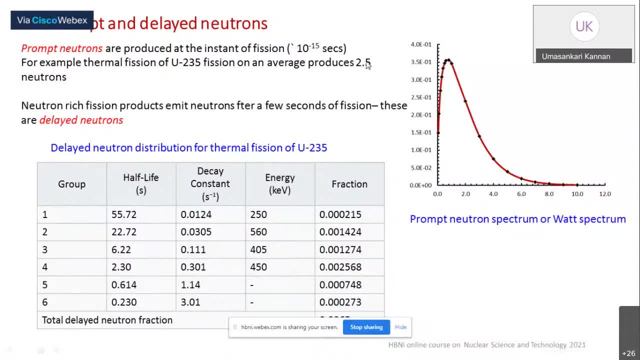 neutrons which are being produced as an instant of fission, But also there are some neutrons which are going to be produced after some time. Like I told you, you saw that lanthanum and bromine were two fission products. So these fission products are neutron rich and they would. 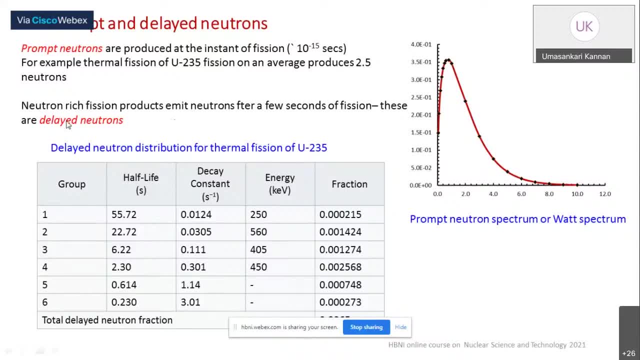 become stable by emitting a neutron. So these neutrons are produced after some time, depending upon the half-life of that particular fission product, And so these neutron-rich fission products emit neutrons after a few seconds of fission. And so all those are different species of fission products. One is that longest half-life. 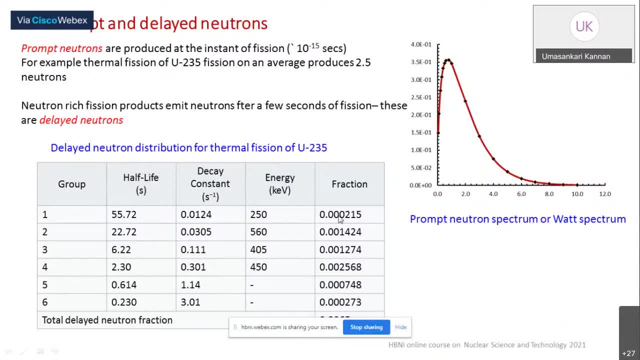 is 50.. Half-life is a neutron, one which gives you about. this is a fraction, and this is the energy of the neutron. Here the energy is about 2 MeV, whereas the energy of the delayed neutron is of the order of KeV. So there is a spectrum here also. So, on an average mode of neutron, fission is going to be. 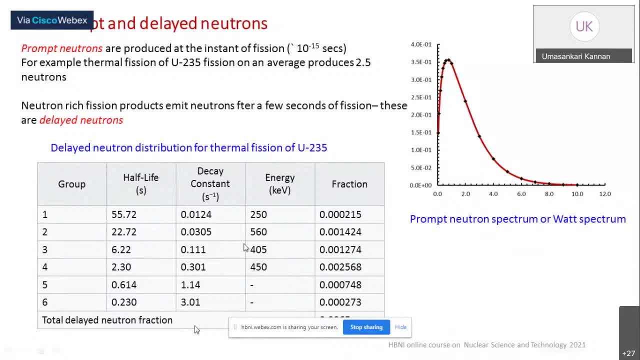 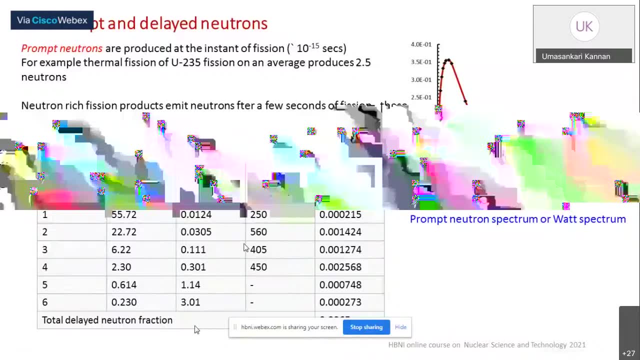 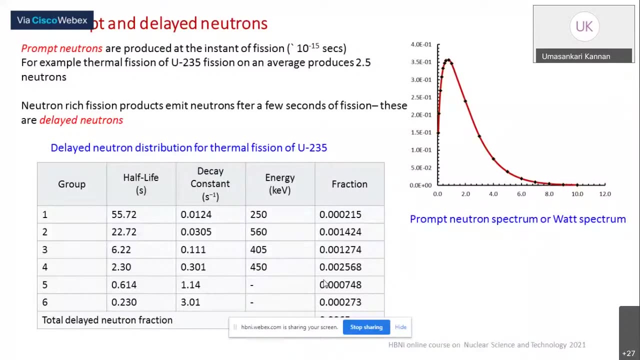 neutron fraction. So 35 is thermal neutron. This delayed neutron fraction is about 0.0065.. So here I wanted to impress upon you There are two neutrons which are at the instant of fission, which is has a, which is, which is emitted at 10, to the power of minus 15. 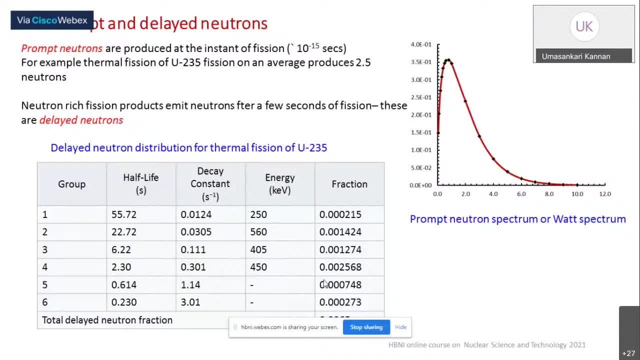 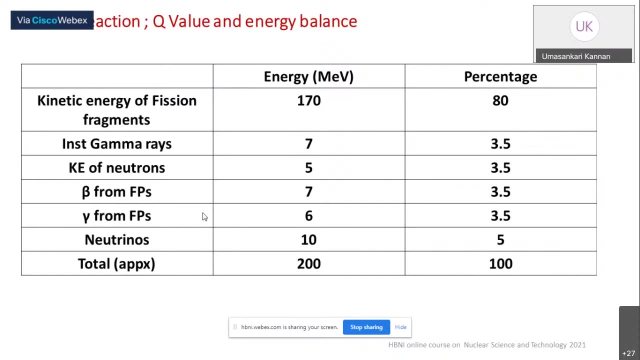 seconds and the delay neutrons which is emitted of seconds after the fission. now let us talk about the energy of the fission. i have told you, on an average, because of the difference in binding energy, we get 200 mev of energy. let us see how this energy is distributed. 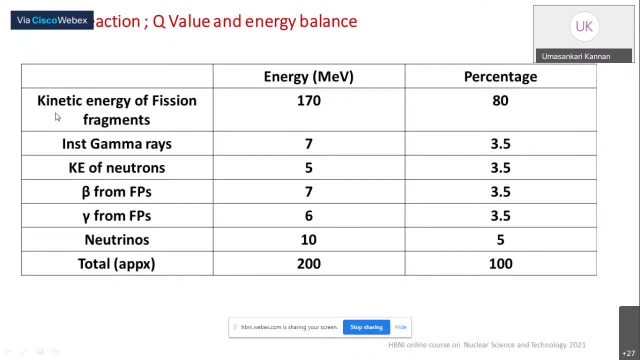 in a fission process. what are all the things which are happening? fission products which are being produced, the fission fragments are moving away in different directions because of the liquid drop of model. liquid drop model. you see that the two fission products are separating out. 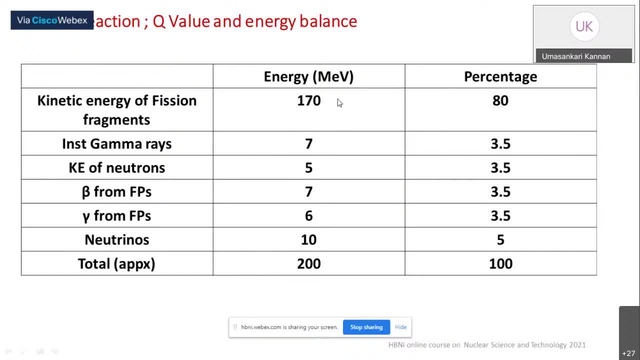 so the kinetic energy of the fission fragment will carry away most of its and most of the energy, that is, people, of the energy pretty efficient, efficient which are being produced. this is around seven mev, the kind of neutrons also of having kinetic energy. that is around five maybe. 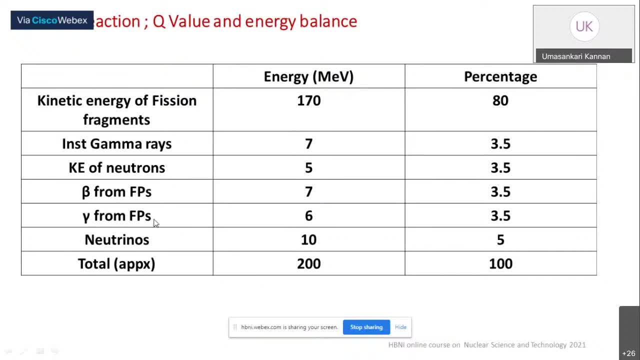 there are betas, neutrinos, then gammas from fission products, betas from fission products. all these are also giving you around seven to six to ten mev, total about 200. maybe is being distributed between these different aspects of the efficient. so the cannon 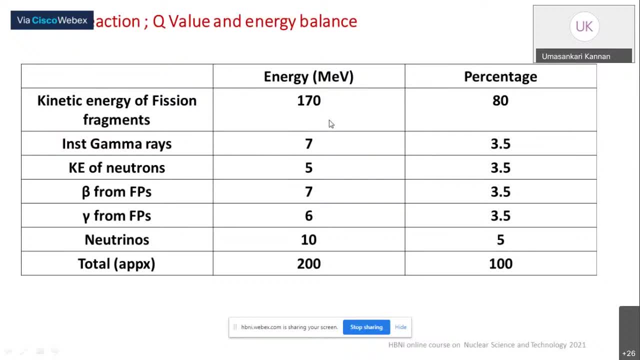 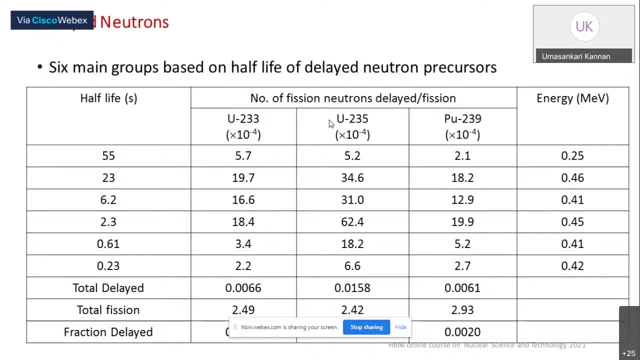 factor of the energy, which is about 170 mev, but this is 200 may be, is called as a q value of the fission reaction. i was telling you about delayed neutrons and then we have categorized the delayed neutrons into different categories based upon its half-life during the fission process. so i don't know about total neutrons as次过比 Mir stock of fission. i think if broad Importance of Fission 2 is quite significant for the fission of the fission and vase candidate energy is two a similar to dergers energy, solız сол is only one. one double component of this felt that the 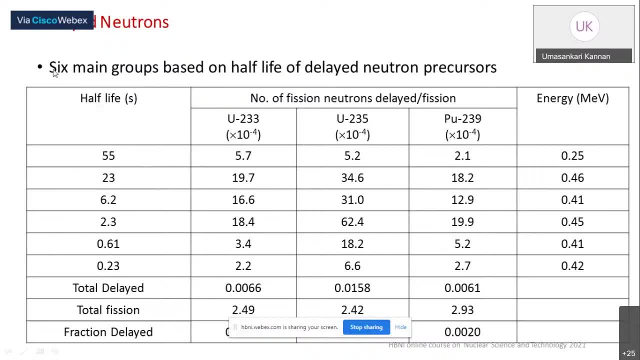 categories based upon its half-life. So in general, we consider six main groups of delayed neutrons which are based on the half-life of the delayed neutron. Now here this is a, and here I try to impress upon you that there are different fissions, which is happening in? 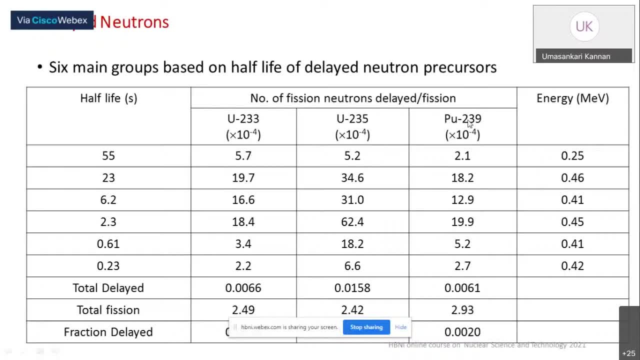 different fissile nuclear. One is uranium-233 or uranium-235 or uranium-239, and the fraction of delayed neutron from the precursor for each of these fissions are going to be different. This is playing an important role in reactor control, which we will learn later. So in 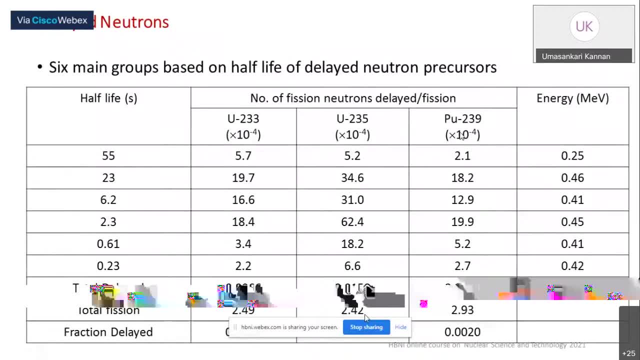 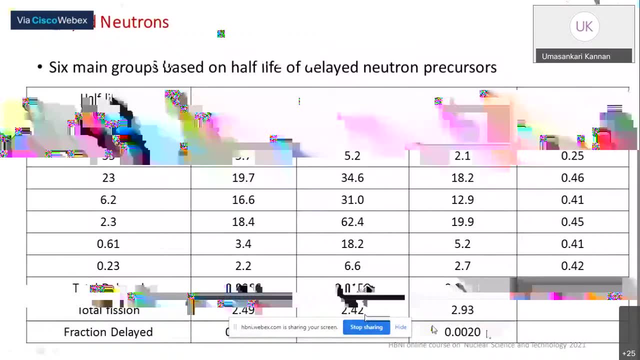 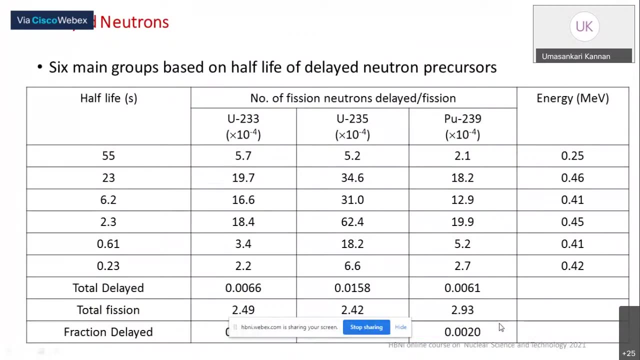 Urative Thermal Equipment. So when plutonium fuel is being used, you have to be very careful in seeing that you do not get a situation where you are not able to control the react. We will come to that a little later. 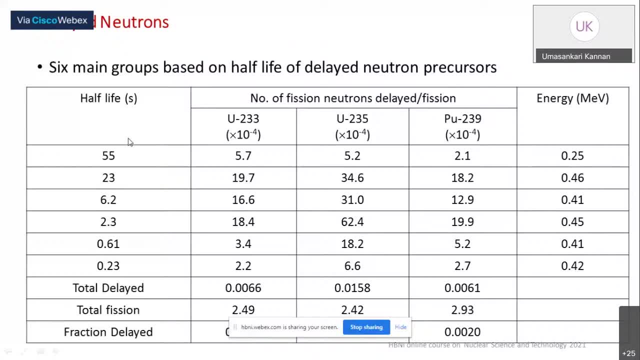 And these are all the energies of the delayed neutron. There is a delayed neutron precursor which is a fission product. These fission products become stable by emitting a neutron And they have an energy particular in the energy levels of the ground state and the 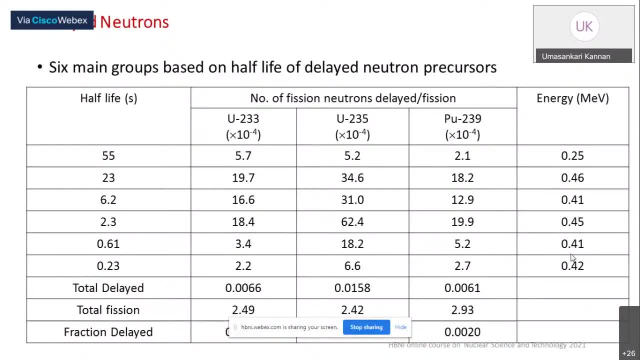 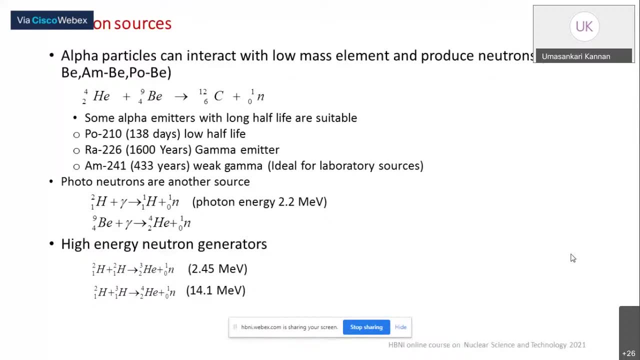 excited state of the fission product. And now we were talking about neutrons. We were talking about the energy inefficient. Now let us talk about: We need neutrons to cause fission, We need neutrons available And we need to produce these neutrons. 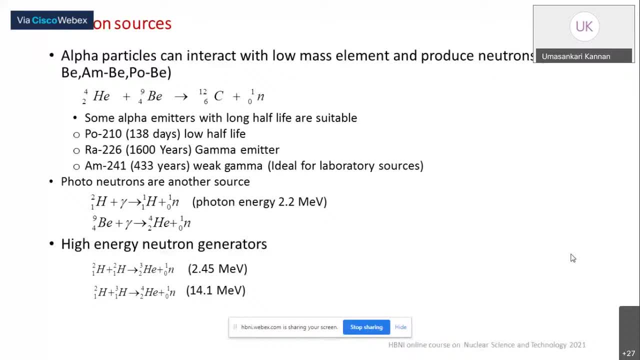 How do we produce these neutrons? See, most important neutrons are the interaction of alpha, So the alpha emitters. they give a neutron in the following, just by the following reaction, cross section reaction. here, For example, there is a radium beryllium, ameritian beryllium or polonium, beryllium sources. 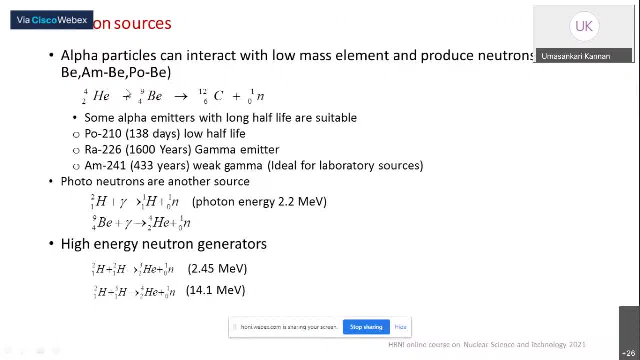 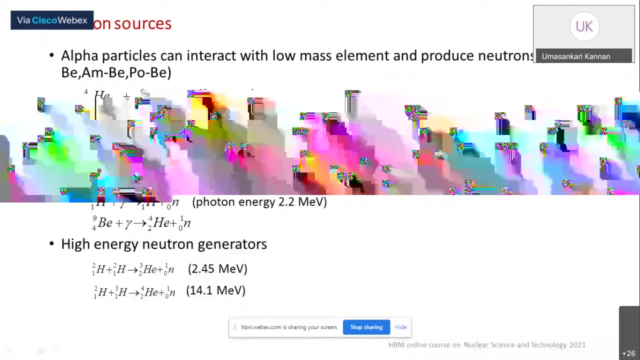 So the alpha, from, From the ameritian, to interact with the beryllium and give away, give a neutron. So this is the reaction which is taking place in for product neutrons. For example, polonium has a 138,, whereas ameritian has 433 years. 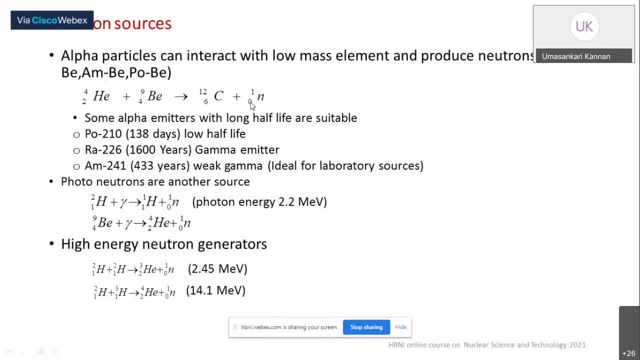 So we generally use an ameritian beryllium source as a source, And these neutrons are also of the order of MAV and they have a spectrum of course. So this ameritian alpha particles interact with low mass element and produce neutrons. 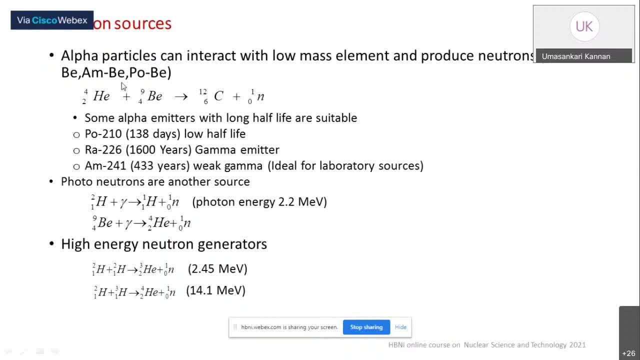 So these are the different types of neutrons which these are different types of neutron sources which can be used some times for a reactor stack Initiate. It is another source of neutrons. For example, gammas. Gammas may interact with deuterium, give away a proton and a neutron. 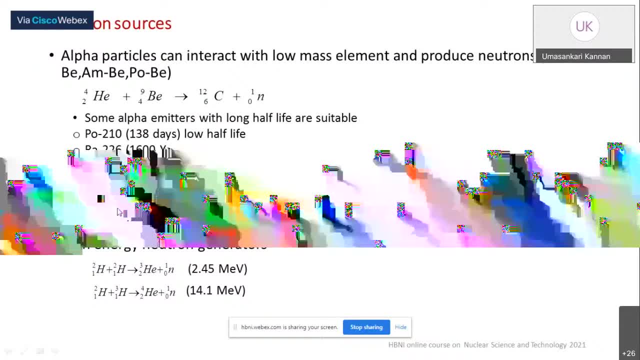 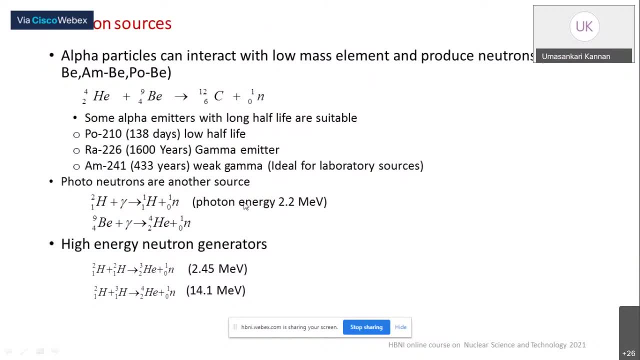 This is a very famous react by which we know that to have a 2.2 MeV of energy, only then it can break the deuterium bond and thereby So this photon energy has to be a 2.2 MeV and we get a neutron of this neutron from. 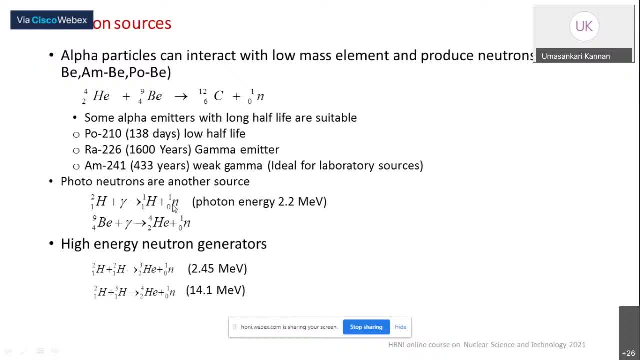 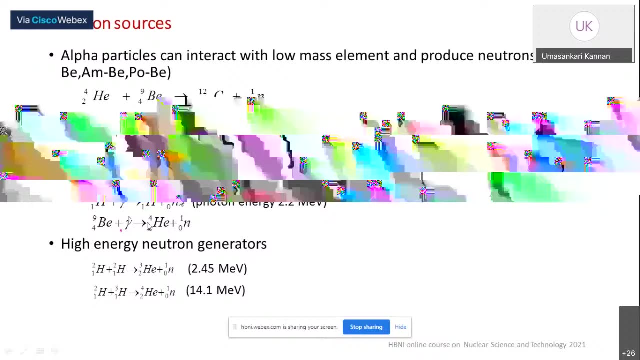 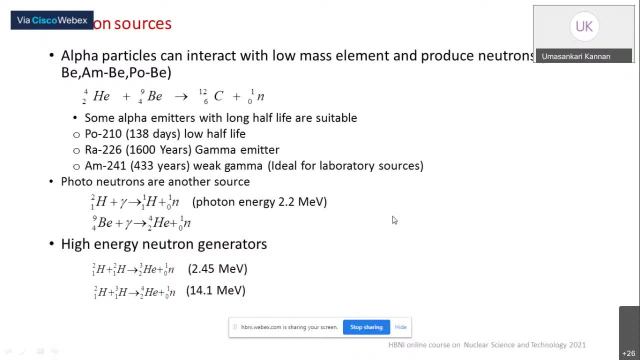 There is another sort of neutron. This is a photo neutron. So these are some alpha and reaction based… gamma and reaction based neutron…. but also there are some high-energy neutron generators Which is based on fusion, For example. For example, DT generators and DD generators. two deuterium atoms together give a helium-3 atom. 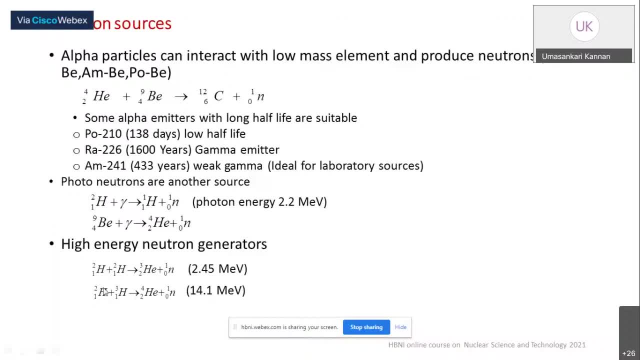 and a neutron of 2.45.. Anyway, this is a famous fusion reaction. Similarly, this fusion reaction can be used as a generator of neutrons, of high-energy neutrons. Similarly, there is a DT fusion, that is, deuterium and tritium. they will interact, they will fuse together. 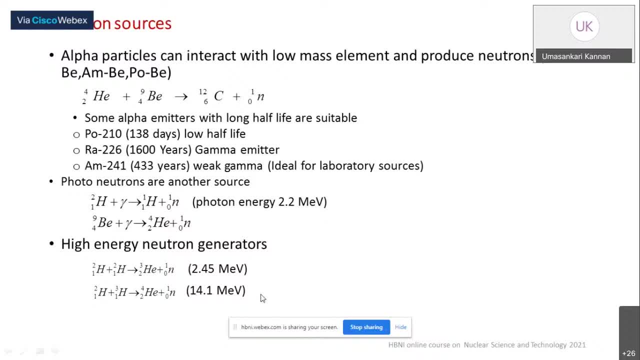 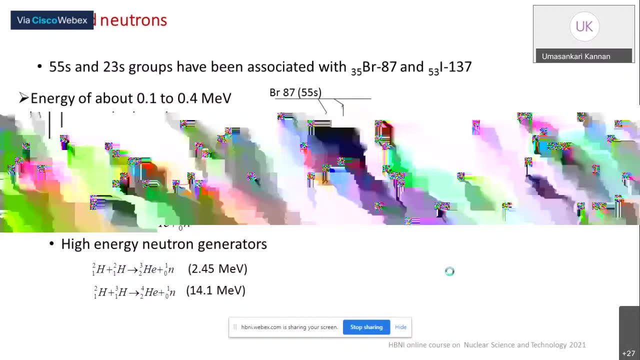 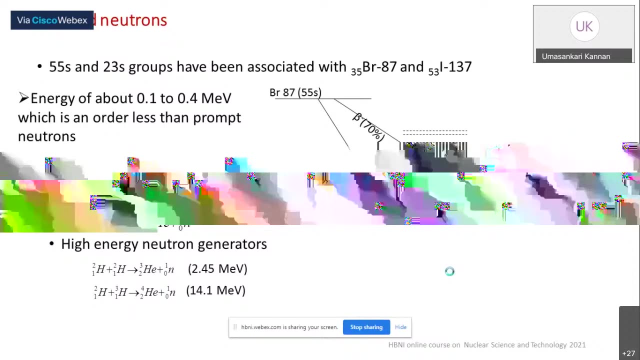 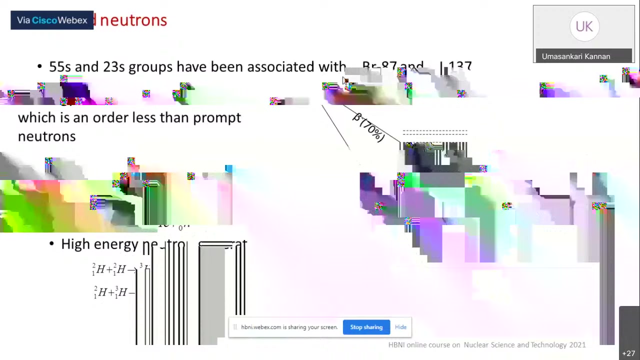 to give a helium and a neutron of 14.1 MeV. So these are high energy neutron generators. Now I was explaining something about there is a seconds and then it would decay to krypton itself by emitting a neutron. this neuron is the energy. 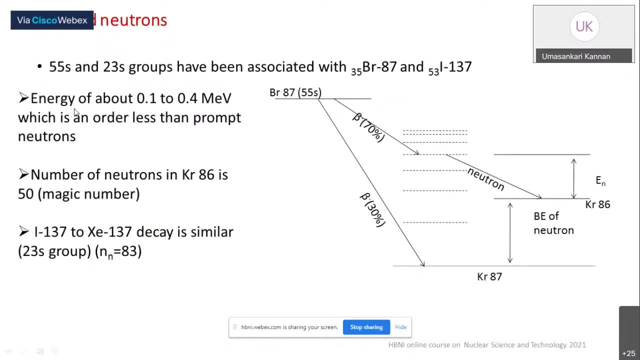 of the krypton 86, 87, and so energy of about 0.1 to 0.4 mev, which is an order less than that of a prompt neutrons, is being generated. and why it goes to krypton? because it's a magic number. it. 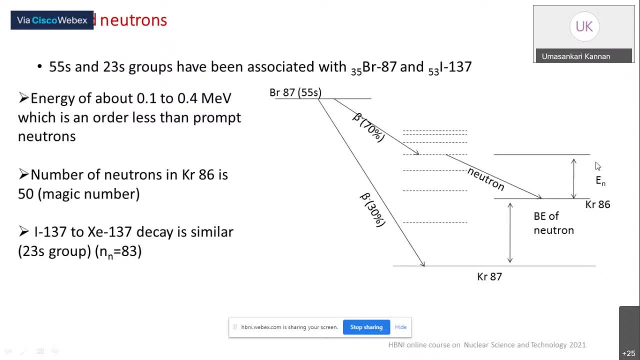 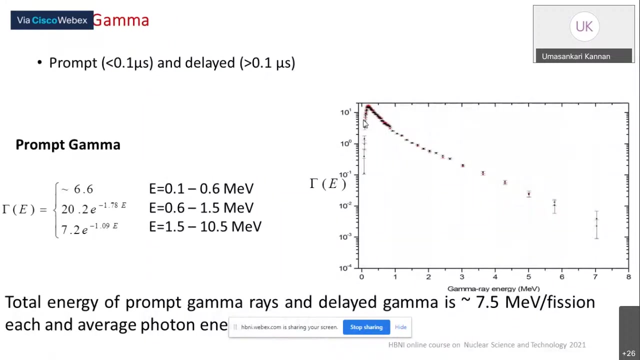 will become? it would like to become stable and come to a stimulation you could dictate to that product: isotope. so basically what? these are the how the delayed neutrons are produced because of the neutron rich fission products. similarly, i will just talking to you about fission gammas. there are 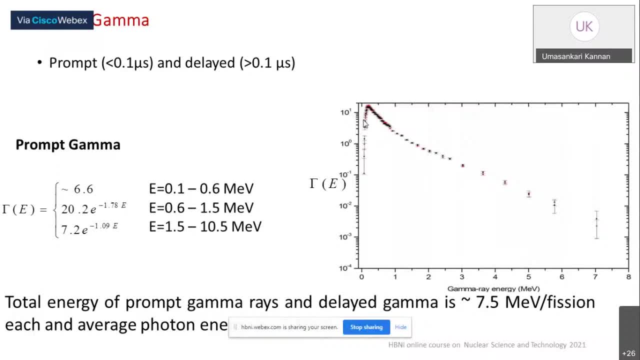 which are being produced in this- gamma rays and delayed gamma rays- is about 7.5 mev per fission, so it has some sort of spectrum like this. so then there are gammas which are being produced in fission, there are neutrons which is being produced in fission there. 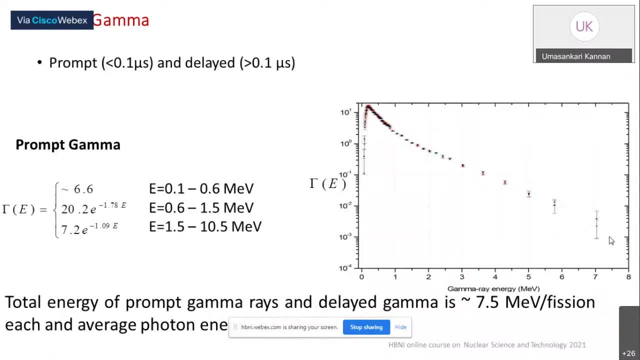 are neutrinos, there are beta particles. all these things are produced in fission. so we bother about these neutrons and gamma because we need to track the electrical energy, energy or your water and or your moderator and so on. so we should take care of these things and we 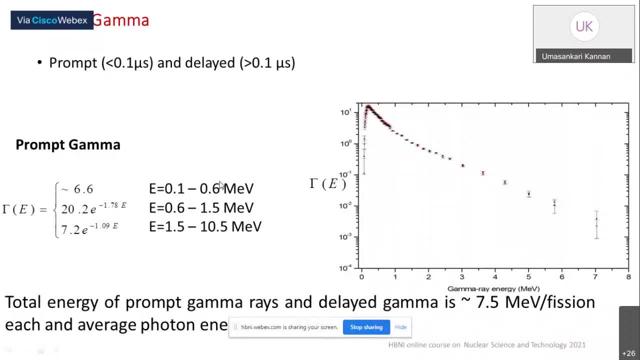 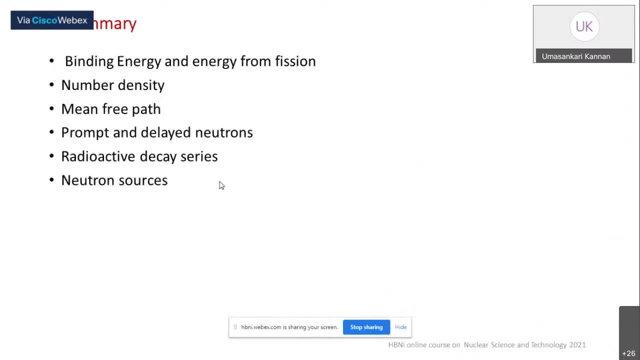 should account for the amount of heat which is being produced by the efficient gammas and the efficient products and the efficient product b and the particles. what is the mechanism of fission? what is the meant by number density? what is meant by mean free path of interaction and how the prompt neutrons and delayed neutrons? what is the? 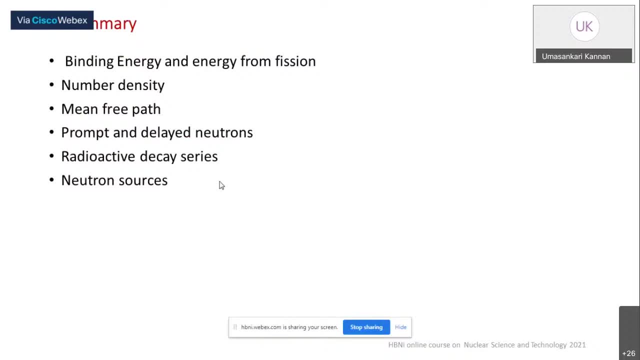 difference between the prompt neutrons and delayed neutrons. how are they produced, then? why some nuclears are radioactive and why some are not radioactive and why some are open. what is the decay? how modes by which they decay, that's alpha, beta or gamma, what we have. 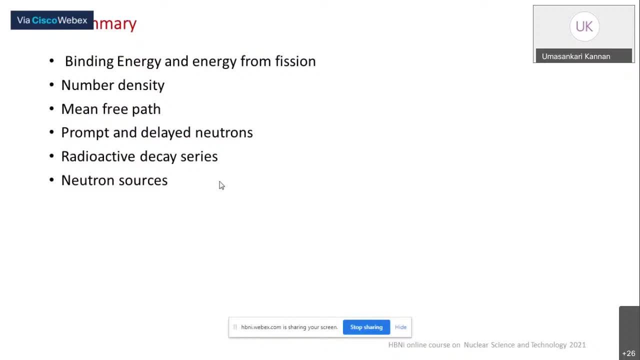 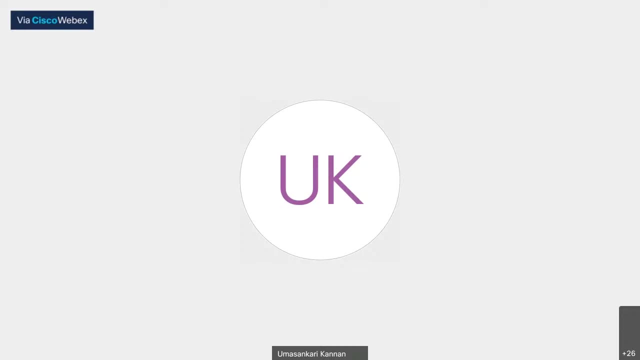 these neutron sources can be used to produce neutrons, so i think i would stop sharing. let me see whether my video is coming and if any questions of any ways asking you can just pose it. uh, so can you hear me now? yes, ma'am, we can hear you. yes, ma'am. 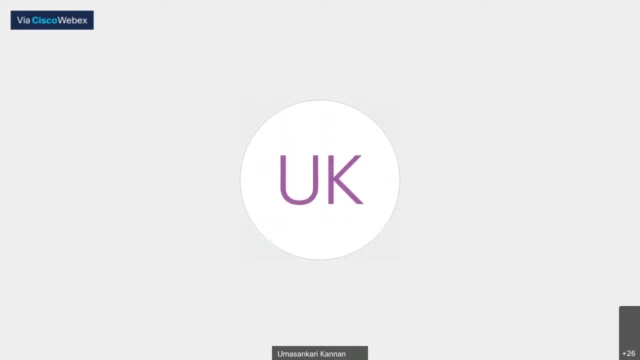 can you hear me? yes, ma'am, we can hear you. yes, okay, are you having any question? was it was my lecture audible on the? was my lecture clear? yes, ma'am, it was clear and it was audible until now. no questions, okay, so there was some. so, yes, ma'am. 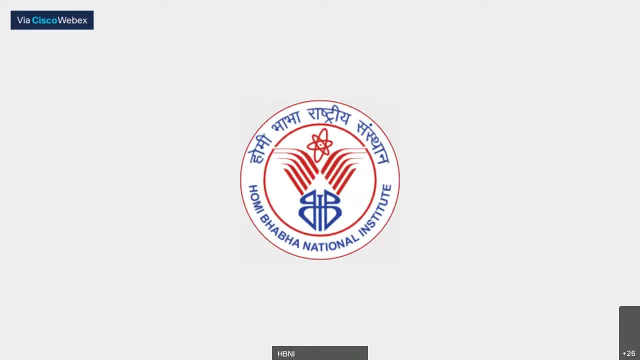 ma'am, no question yet. okay, let us try to rectify this in my next lecture, but i would leave my presentations in the website so that you could go through it and then when you do some. but i this was a recap of your nuclear physics lectures which you might have heard.